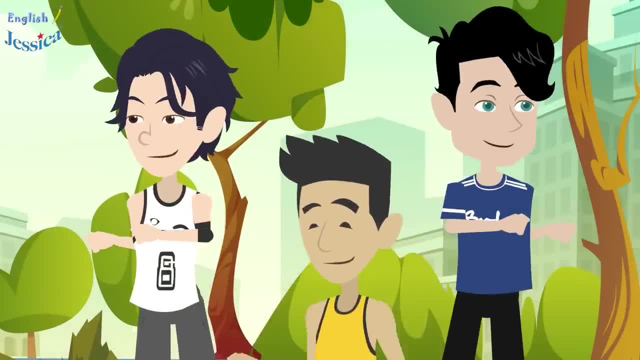 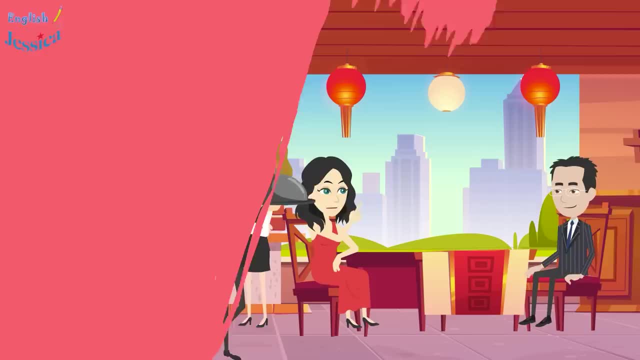 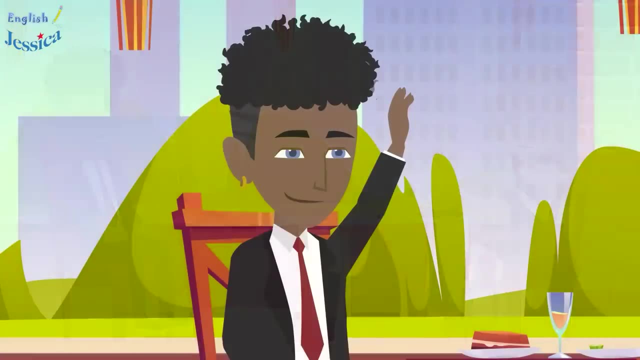 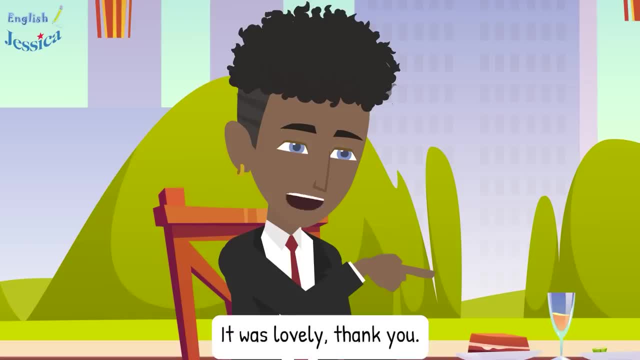 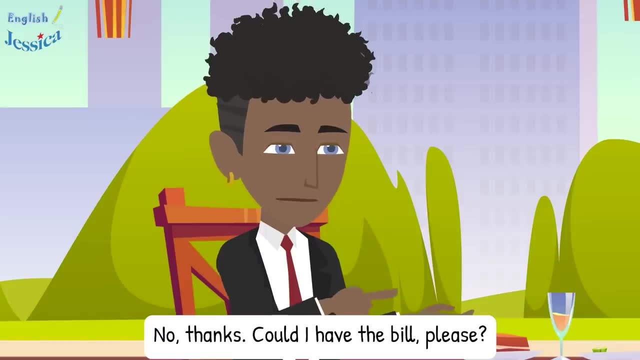 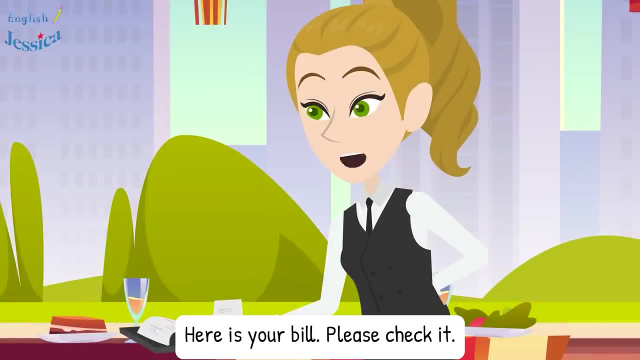 How was your meal? It was lovely, thank you. Is there anything else I can help? No thanks, Could I have the bill please? Sure, sir, Please wait a moment. I'll bring you the bill. Here is your bill. Please check it. Okay, let me see. 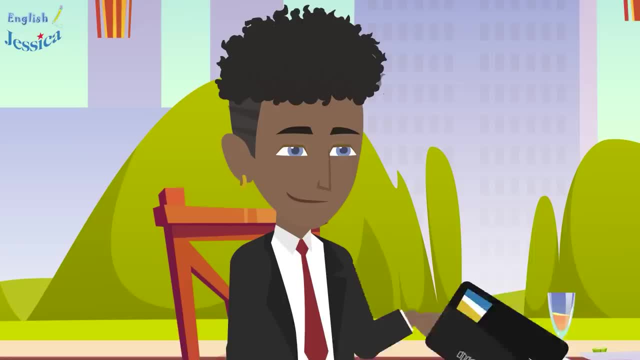 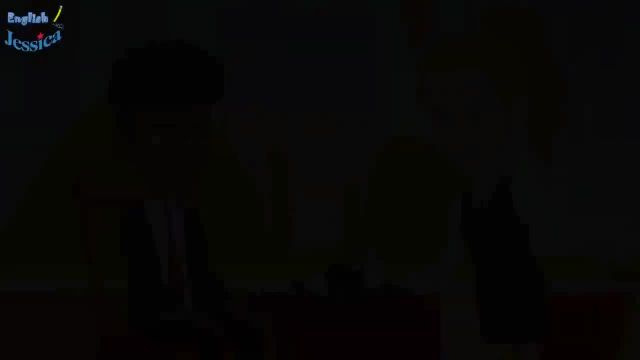 Yes, no problem. Do you want to pay now? Yes, here is my card. You can take it. Great, Okay, Thank you. Thanks, sir. Please wait a moment. Everything is done. Here is your card and bill. 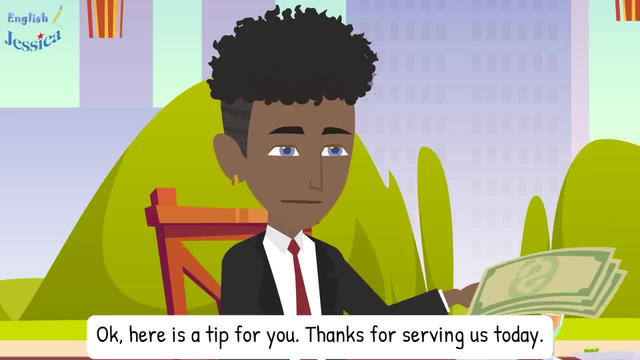 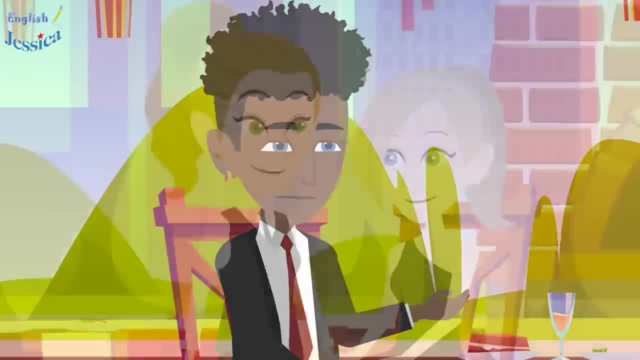 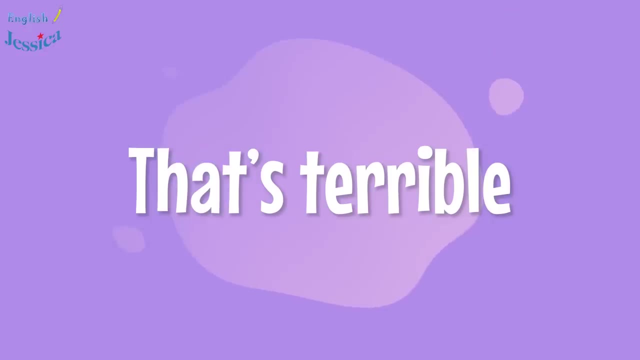 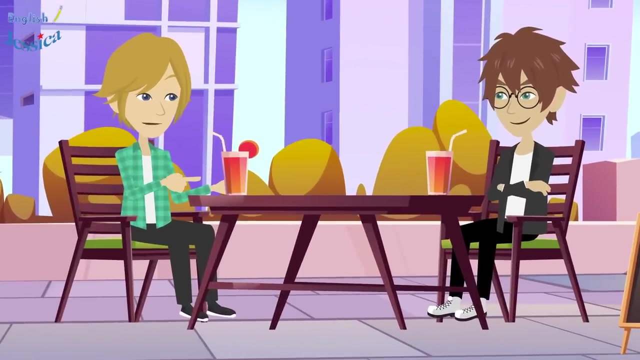 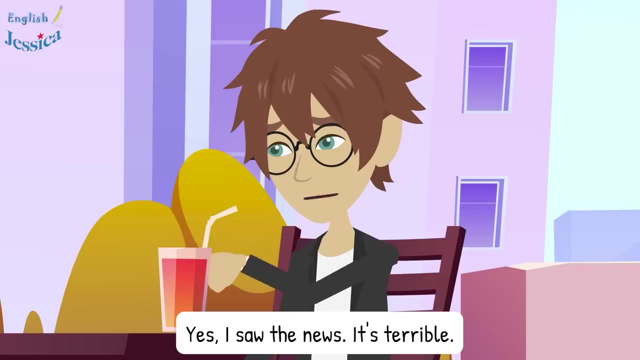 Okay, Here is a tip for you. Thanks for serving us today. Thank you very much, sir. I hope you had a great time tonight. Thanks, That's terrible. Have you heard of the tornadoes last night in Kentucky? Yes, I saw the news. It's terrible. 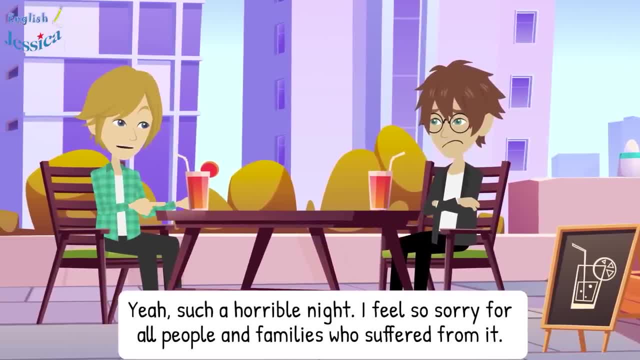 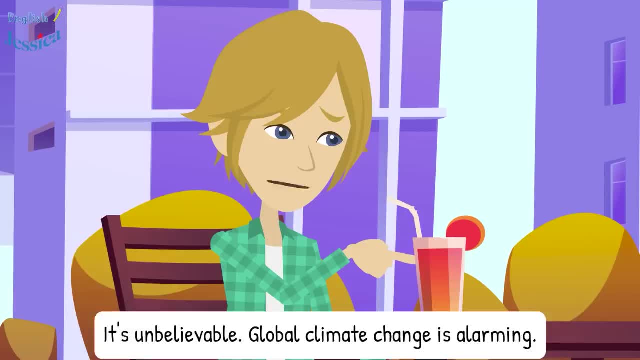 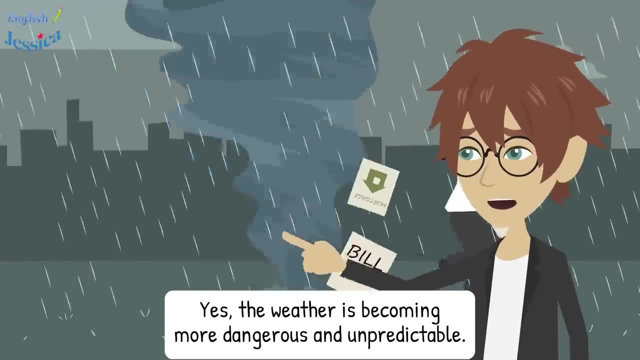 Yeah, such a horrible night. I feel so sorry for all people and families who suffered from it. It's so crazy weather, It's unbelievable. Global climate change is alarming. Yes, the weather is becoming more dangerous and unpredictable. Do you know anyone living in the area? 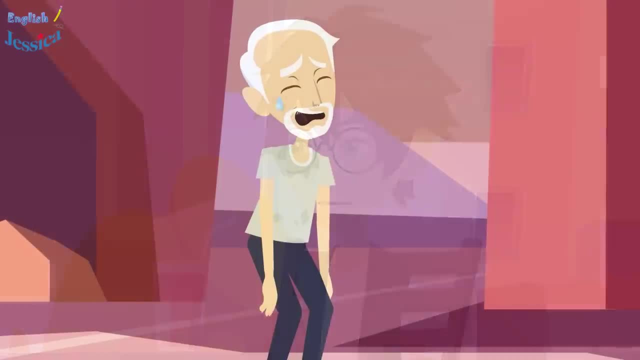 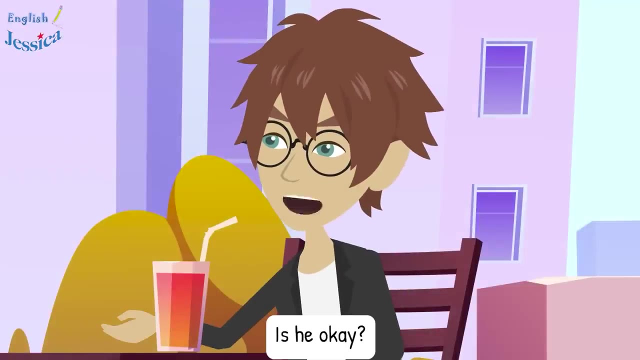 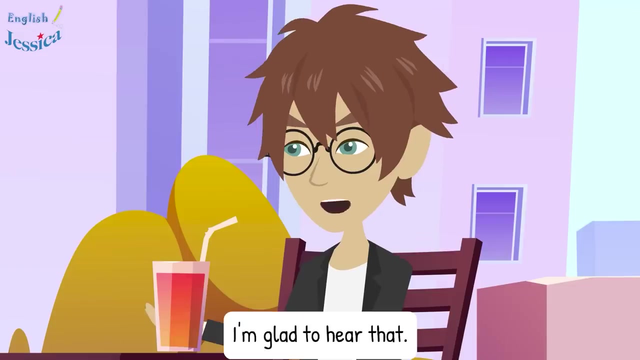 No, I don't. How about you? Yes, not in Kentucky, but I have a relative living in that area affected by a tornado. Is he okay? Yes, fortunately He and her family are safe. I'm glad to hear that. 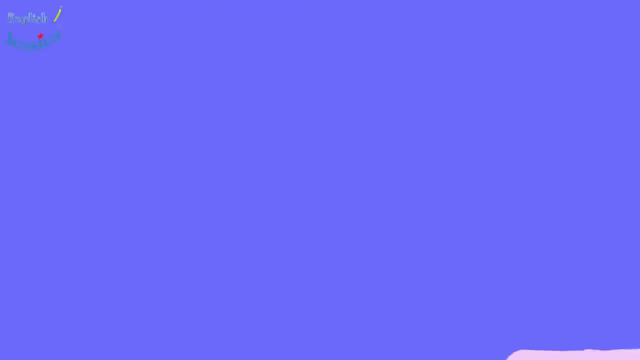 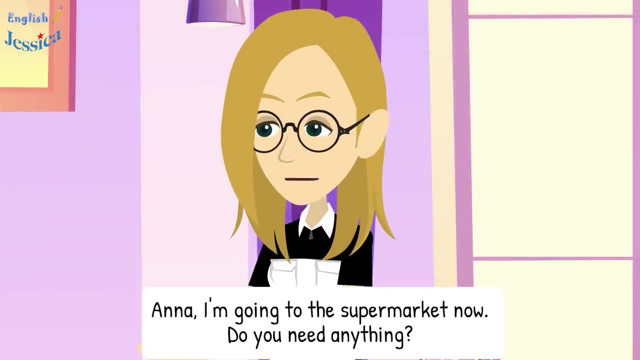 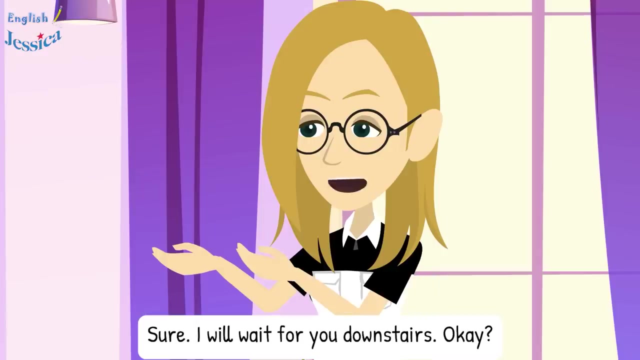 I'll be there in 10 minutes. I'll be there in 10 minutes. Anna, I'm going to the supermarket now. Do you need anything? Oh, I want to go too. Can you wait for me a bit? Sure, I will wait for you downstairs, okay. 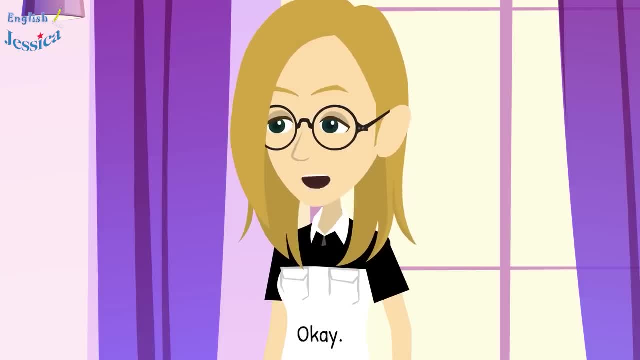 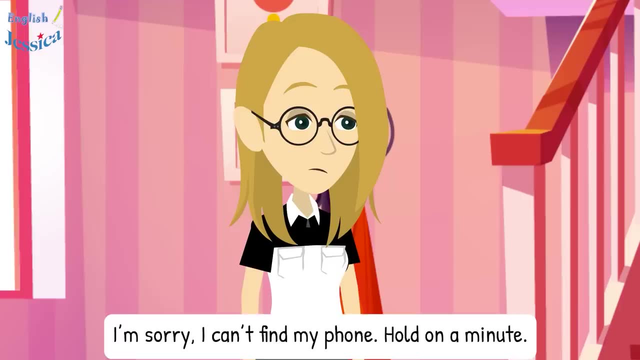 Yes, I will be there in 10 minutes. Okay, Anna, are you ready? Yes, I am. I'm sorry I can't. oh no, I didn't mean to. I'm sorry I can't. oh no, I didn't mean to. 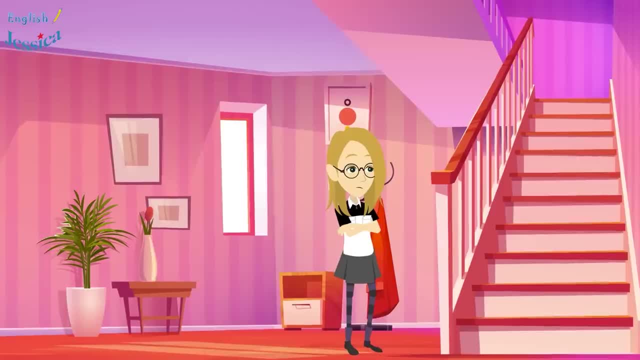 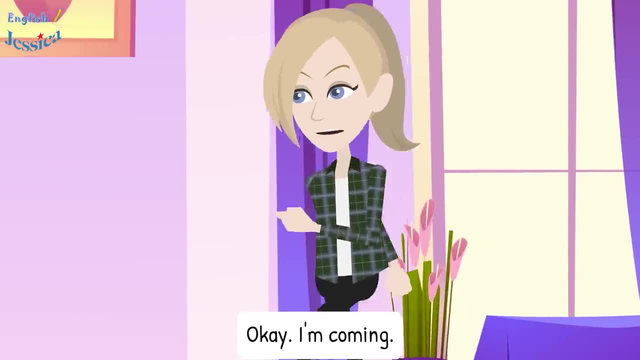 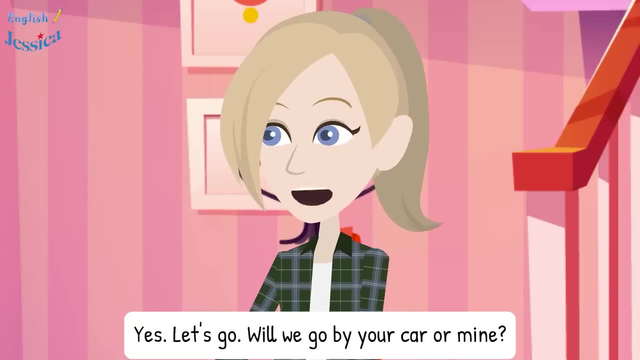 I can't find my phone. Hold on a minute. Do you need me to help you find it? No, I'm good, Be quick. Okay, I'm coming Ready. Yes, let's go. Will we go by your car or mine? My car, It needs. 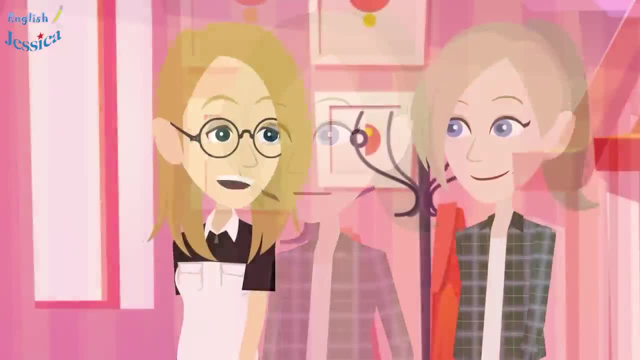 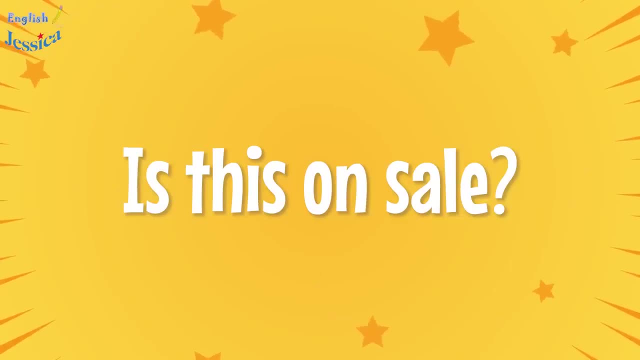 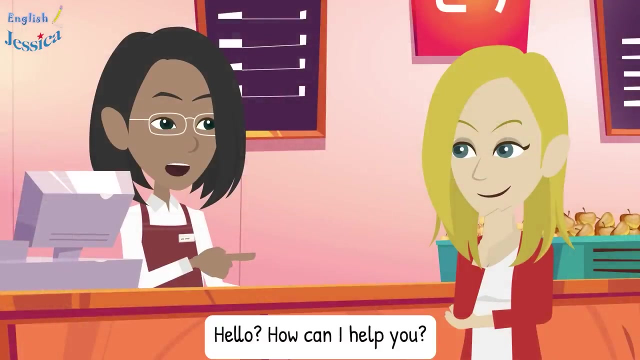 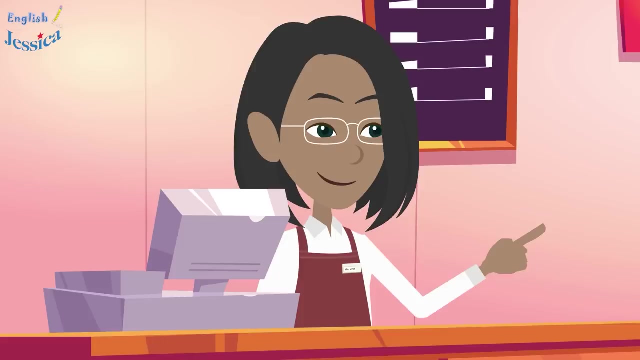 to be refueled. Okay, Is this on sale? Hello, how can I help you? I would like to buy some flour, apples and cheese. Do you have them? Yes, we have. What kinds of flour do you need? 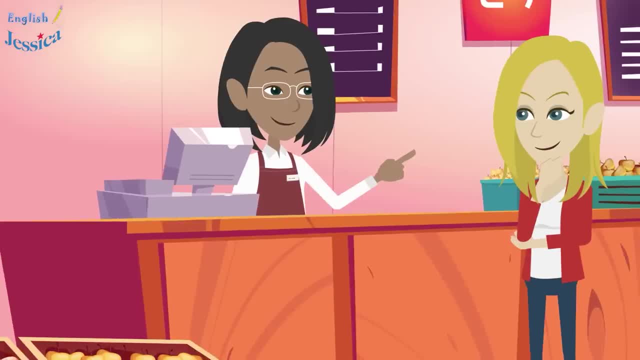 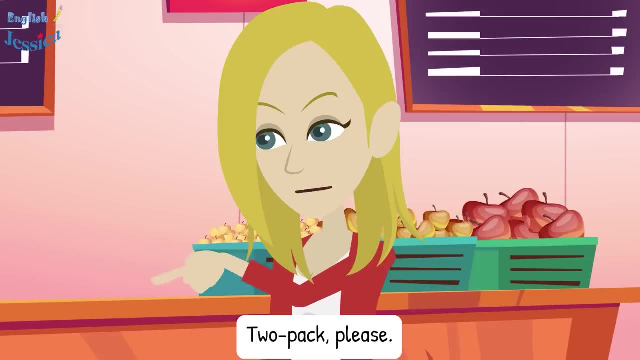 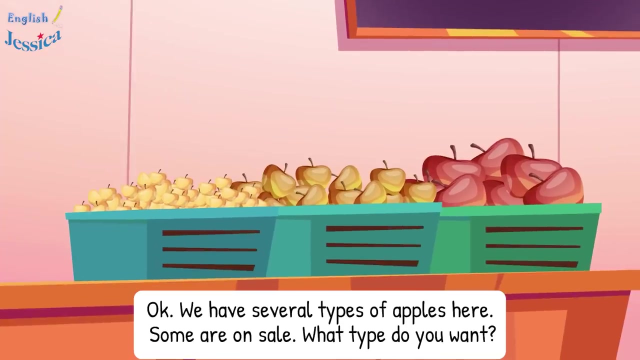 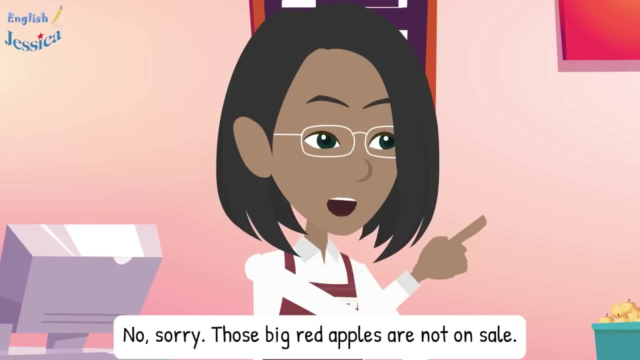 I want to make apple pie. Ah, then you will need all-purpose flour. How much flour do you need? Two pack, please. Okay, we have several types of apples here. Some are on sale. What type do you want? Is this on sale? No, sorry, Those big red apples are not on sale. How about? 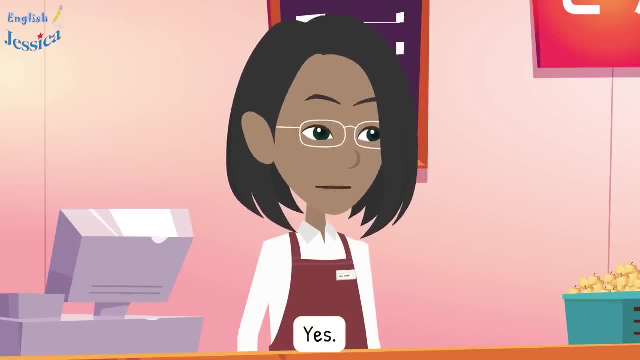 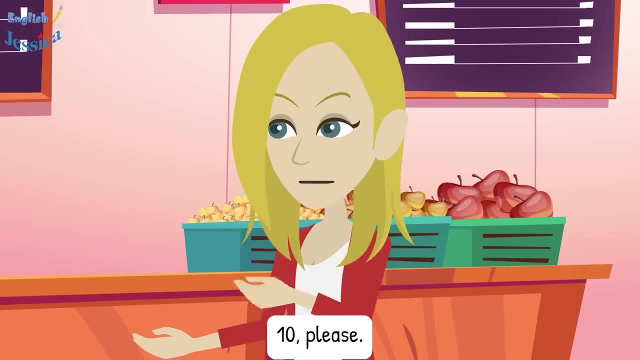 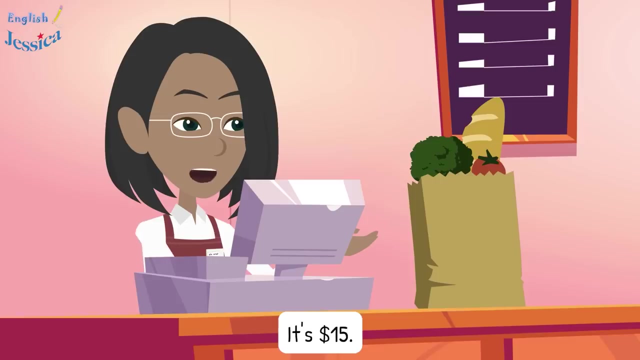 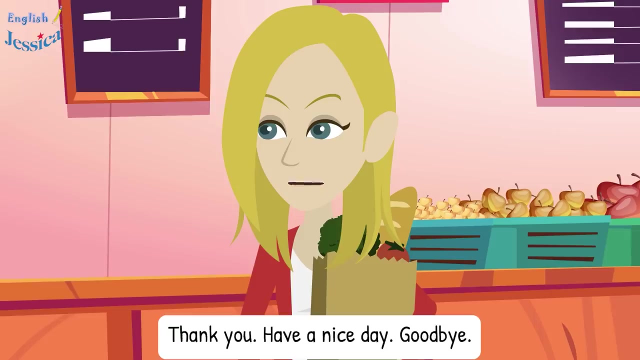 these smaller ones. Yes, I will take these. How many apples do you want? Ten, please. Is that all? Yes, How much is it? It is fifteen dollars. Here you are Done. here is your receipt. Thank you, Have a nice day, Good-bye. 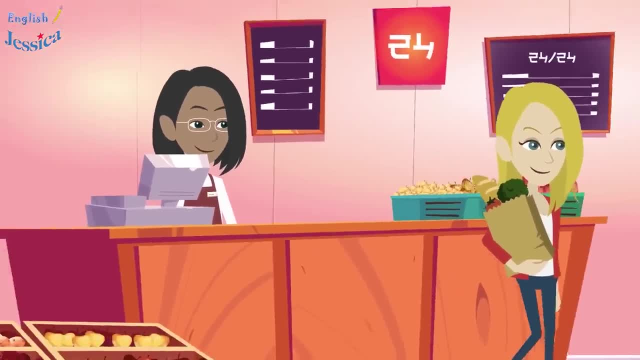 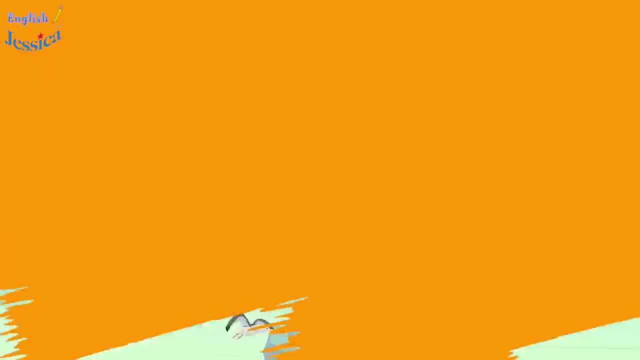 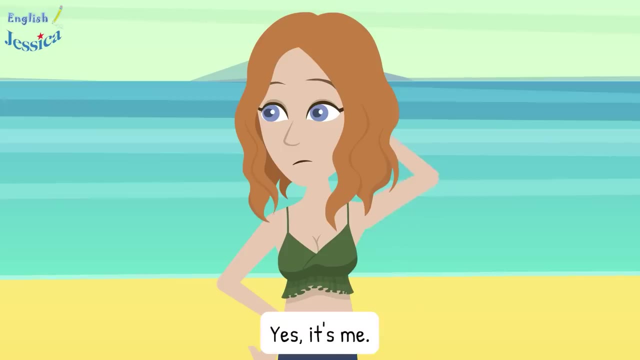 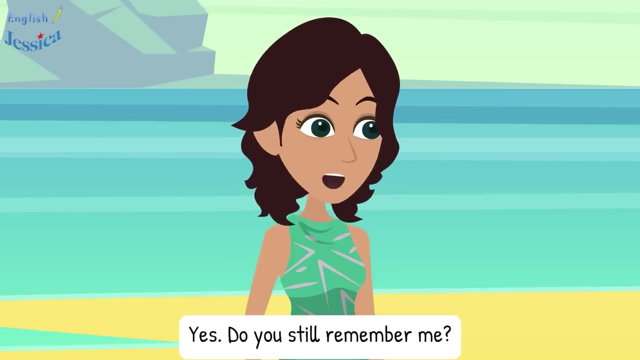 Thank you, You too. 10 minutes later, Are you ready? Yes, I am. Let's grab a coffee sometime. Lily, is that you? Yes, it's me. You are Layla. Layla. Yes, Do you still remember me? 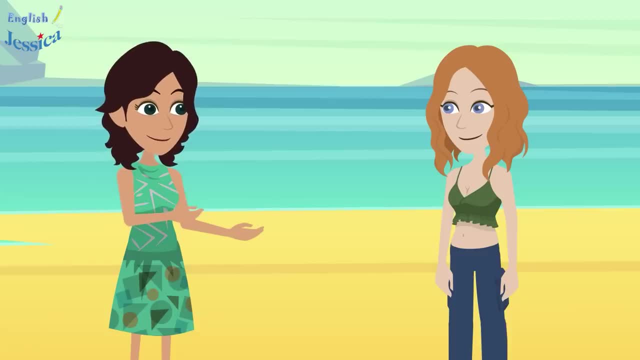 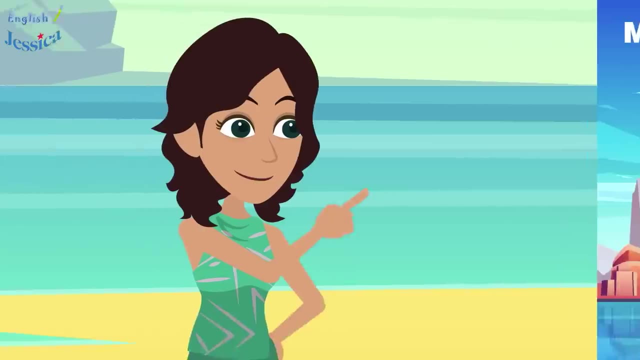 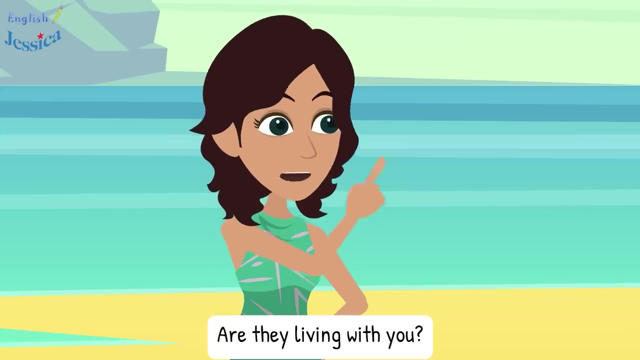 Of course. How can I forget Long time, no see. Where are you living now? I'm living in Michigan now. Really, How are your parents? They're good Thanks for asking. Are they living with you? No, they're still living here. I came to visit them. 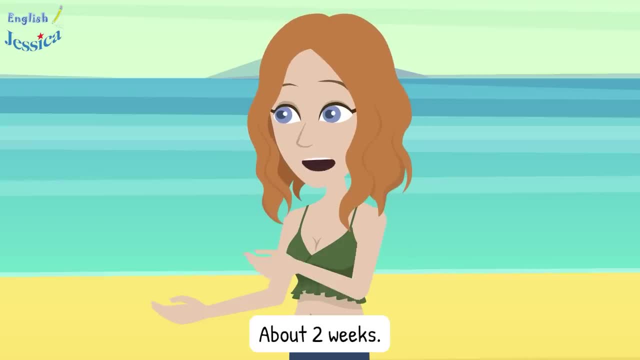 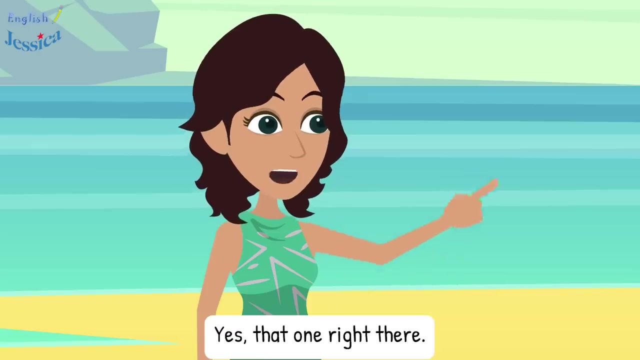 How long will you stay? About two weeks. Let's grab a coffee sometime. Sure, How about this Friday night? I'm good. Do you know any good cafe here? Yes, That one right there. Oh, nice Is 8pm, okay for you. 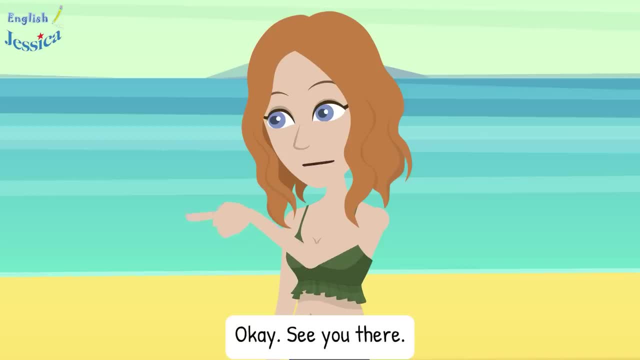 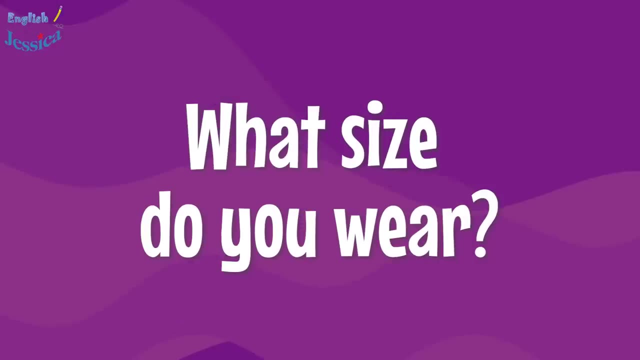 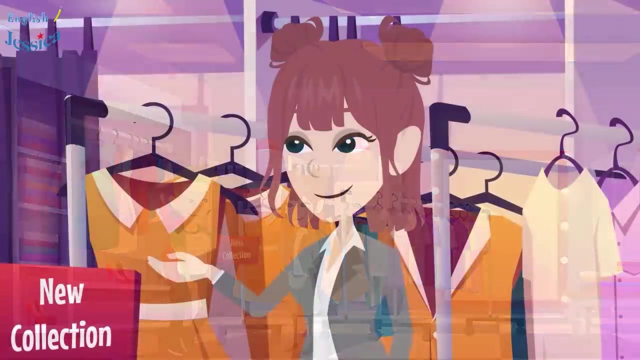 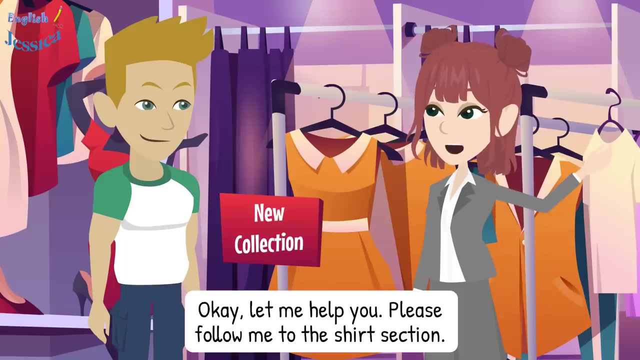 Yes, Let's meet up at 8.. Okay, See you there. What size do you wear, Hi, How may I help you? Hi, I'm looking for a shirt. Okay, Let me help you. Please follow me to the shirt section. 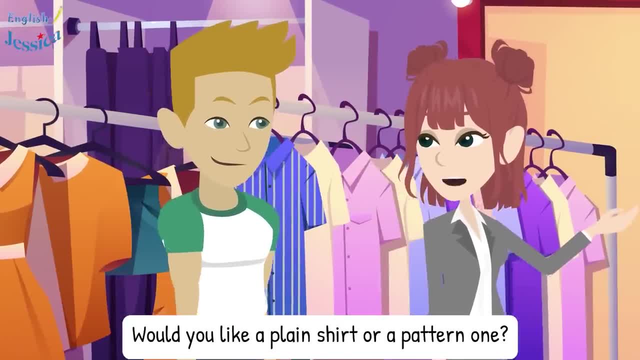 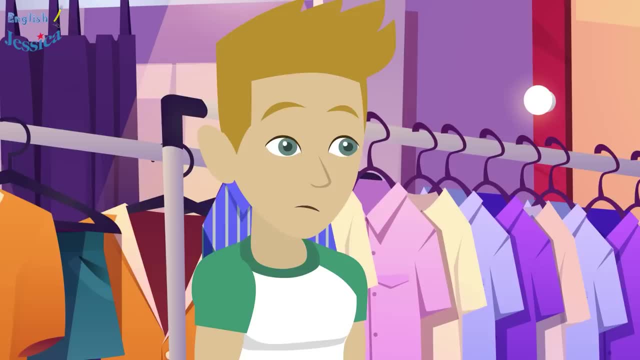 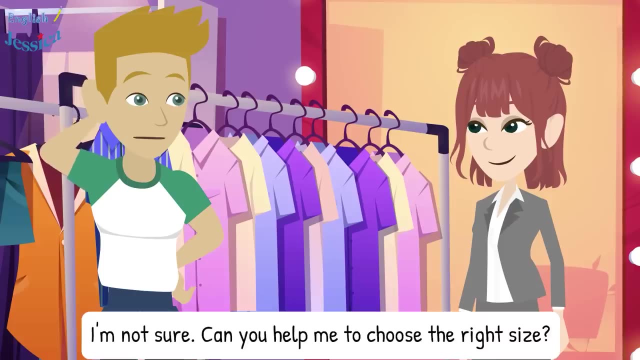 Okay. Would you like a plain shirt or a patterned one? I would like a plain shirt, Any particular color, Blue or grey. What size do you wear? I'm not sure. Can you help me to choose the right size? Yes, May I know your height and weight. 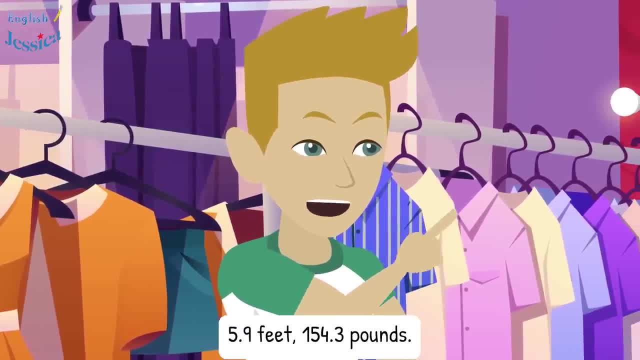 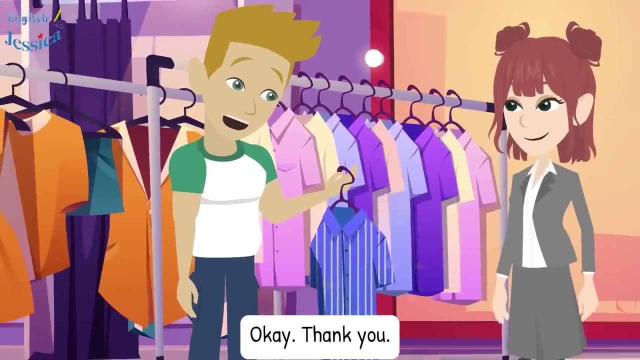 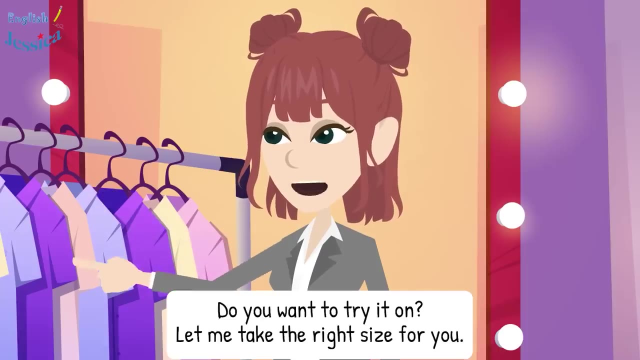 5.9 feet, 154.3 pounds, So let's try this one, Okay, Thank you. Oh, this striped shirt looks good. Do you want to try it on? Let me take the right size for you. Thank you so much. 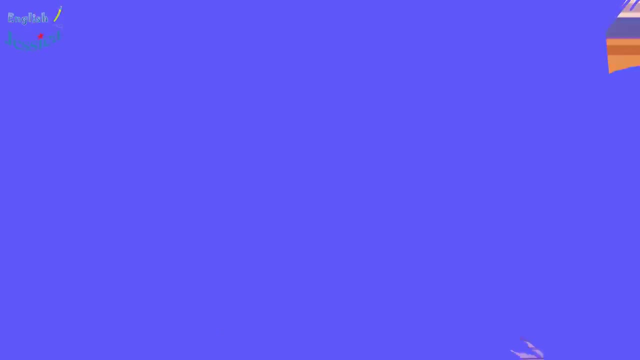 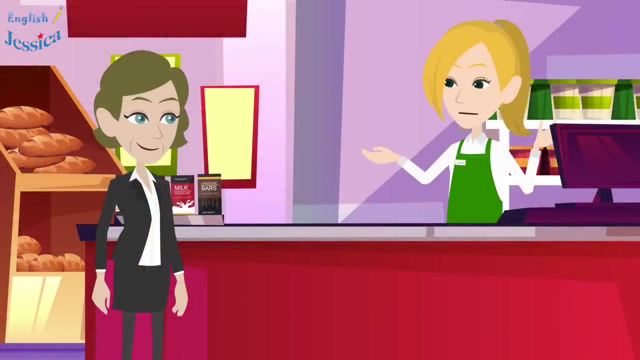 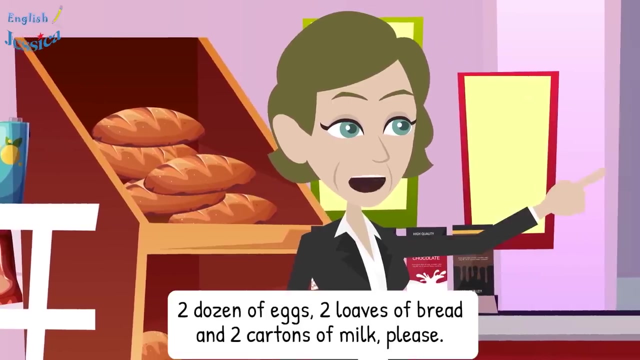 Great, I'll take it. I'm sure you'll like it. I'll wear it. Thank you, Good morning. May I help you? Hi, I would like some eggs, bread and milk. Quantity: Two dozen of eggs, two loaves of bread and two cartons of milk, please. 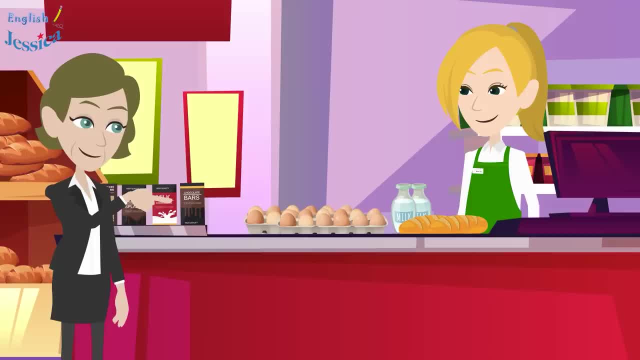 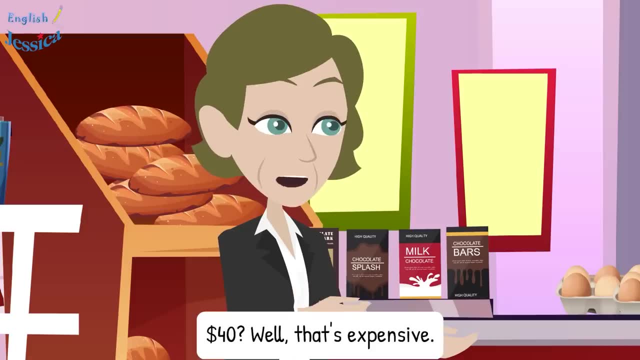 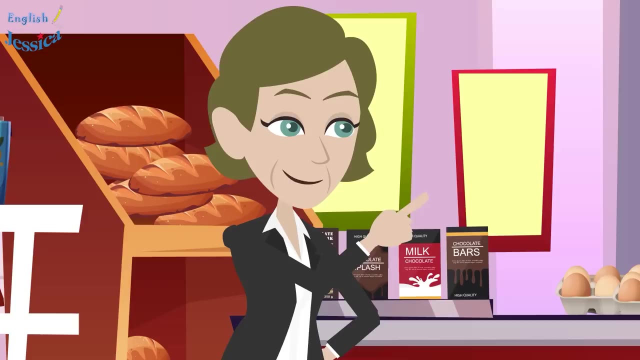 Okay, Is there anything else that you need? Um, how much is this chocolate box? It's $40.. $40? Forty dollars? Well, that's expensive. We have a smaller version here, if you want to try it out. How much is this one? 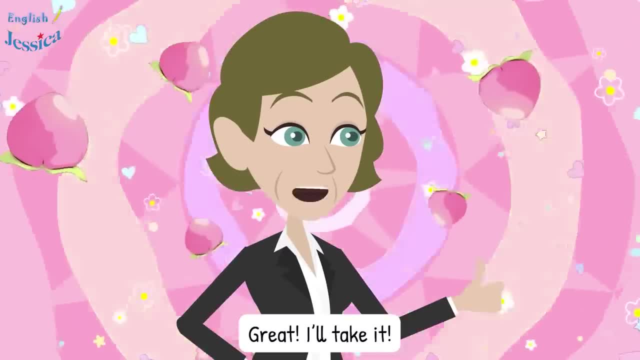 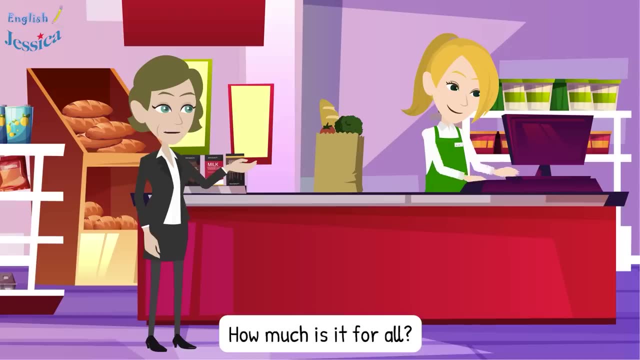 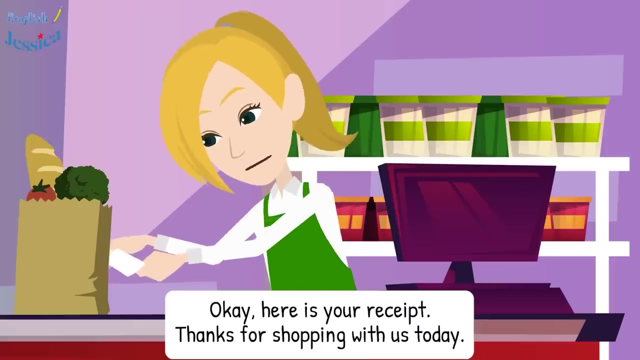 It's ten dollars? Great, I'll take it. Okay. anything else that you like? No, that's all. How much is it for all? It's twenty-eight, seventy. Here you are. Okay, here is your receipt. Thanks for shopping with us today. 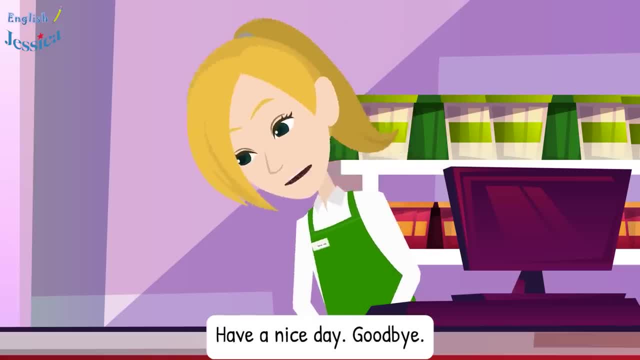 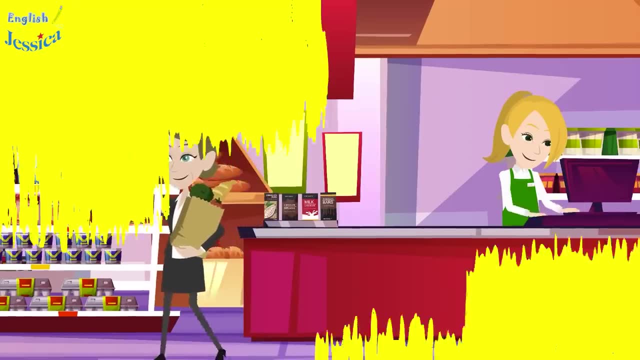 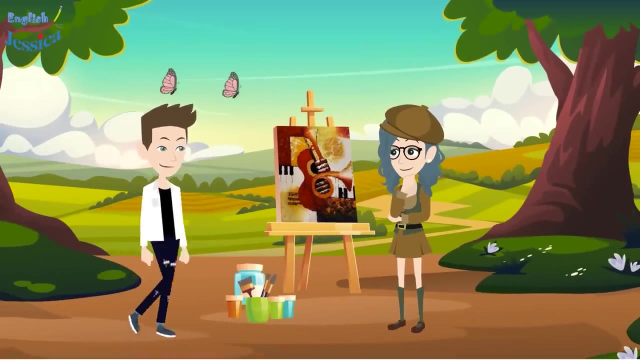 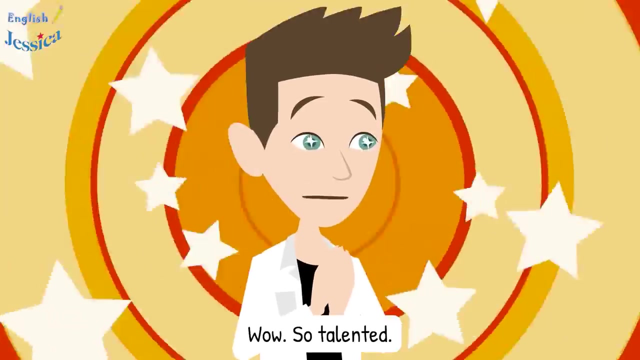 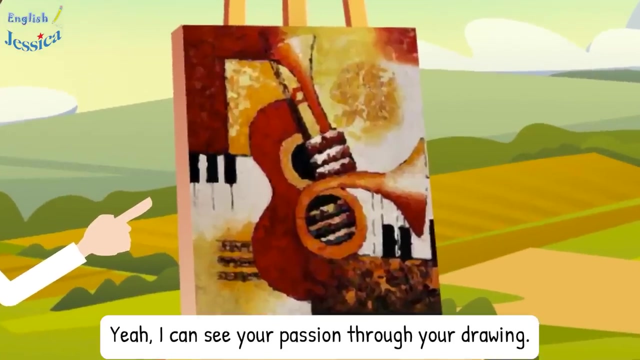 You're welcome. Goodbye, Have a nice day. Goodbye. What kind of art do you like, Jenny? did you draw this picture? Yes, I did. Wow, so talented. Thank you, I really love drawing. Yeah, I can see your passion through your drawing. 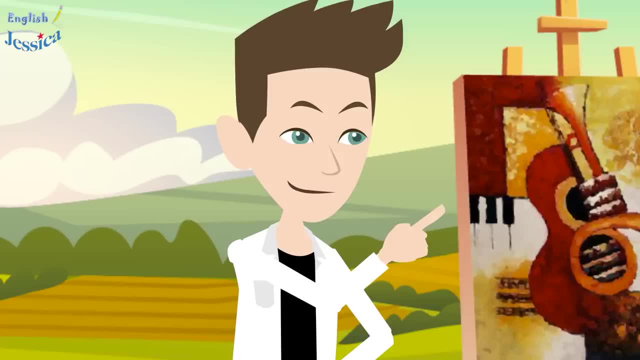 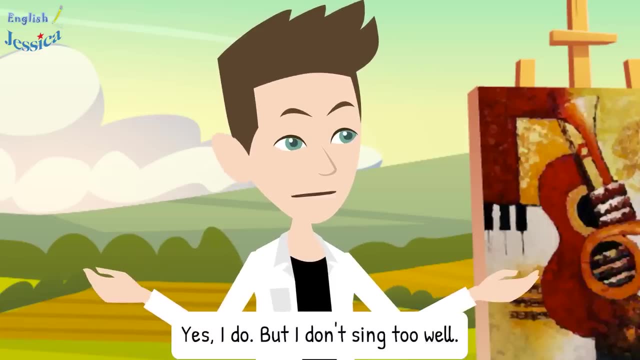 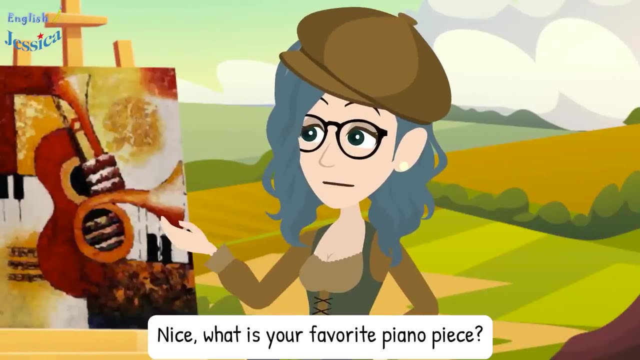 How about you? What kind of art do you like? I like music, Music. Do you like singing? Yes, I do, But I don't sing too well, I prefer playing the piano. Nice, What is your favorite piano piece? 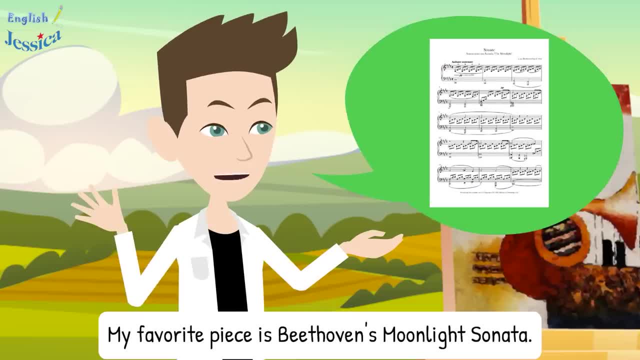 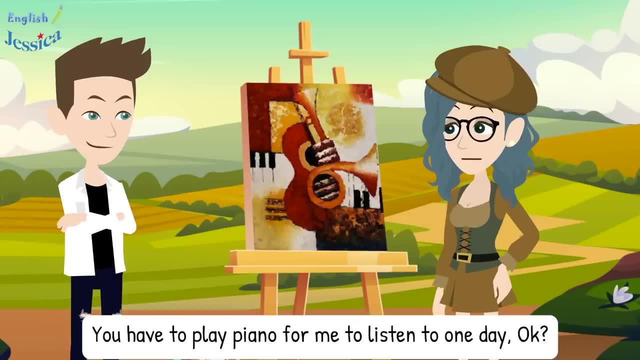 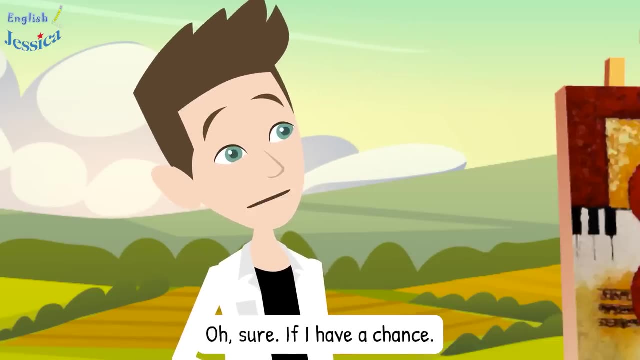 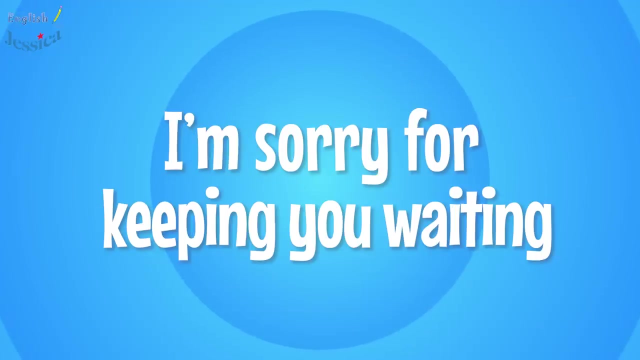 My favorite piece is Beethoven's Moonlit Sonata. Do you like him too? Yes, he is my favorite composer. You have to play the piano for me to listen one day, okay, Oh, sure, if I have a chance. I'm sorry for keeping you waiting. 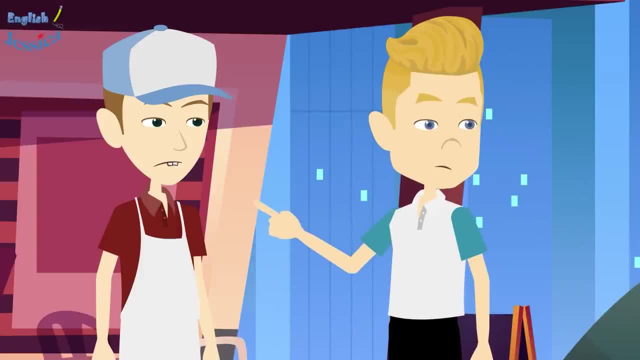 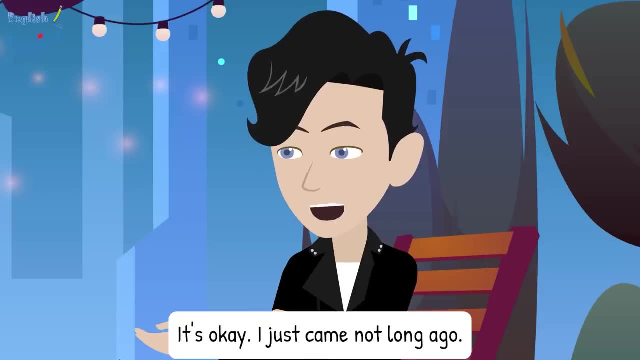 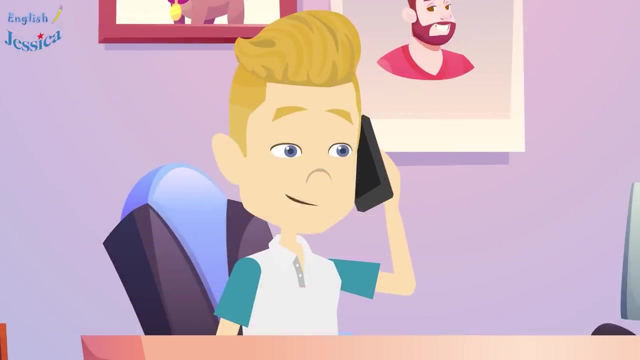 Hi Dan over here. Hi, Josh, I'm sorry for keeping you waiting. It's okay. I just came not long ago. Yeah, I was going to leave work. then I got a client's call. Are you busy now at work? 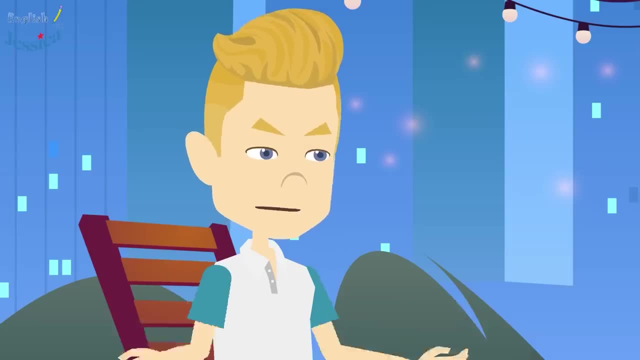 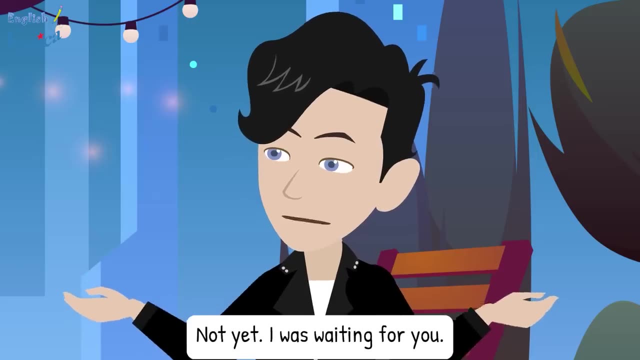 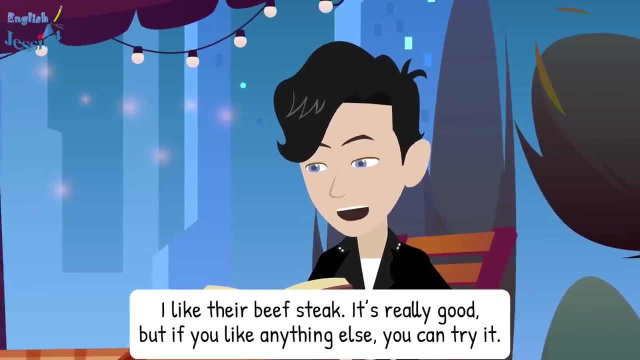 Yes, I am. It's the end of the year, you know. Yeah, especially in your field. Have you ordered food? Not yet. I was waiting for you. Any suggestion? I've never been here before. I like their beefsteak. It's really good. but if you like anything else, you can try it. 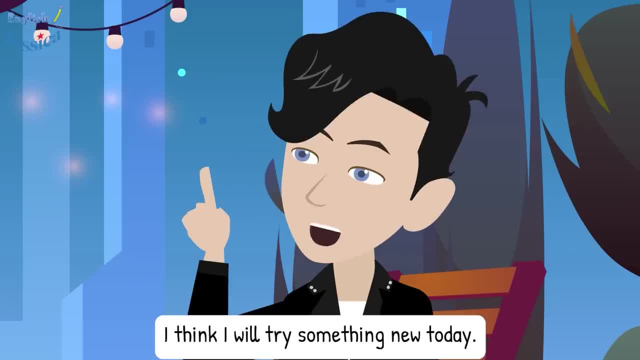 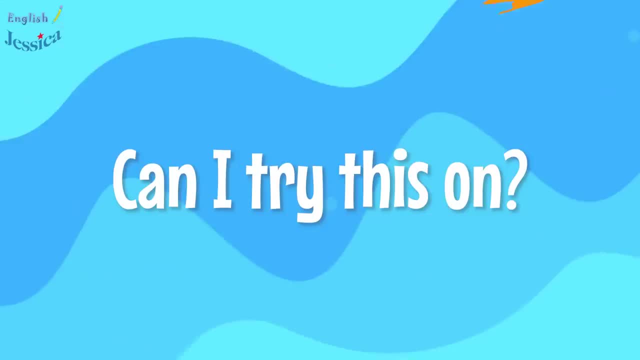 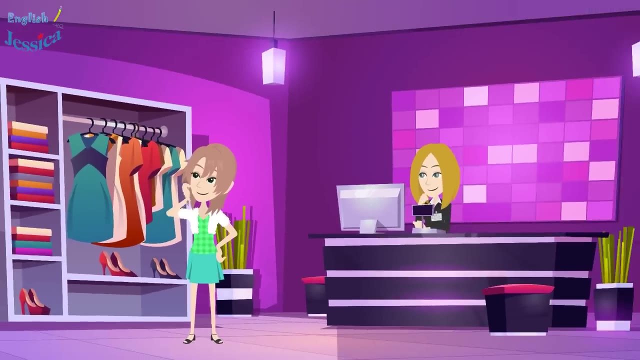 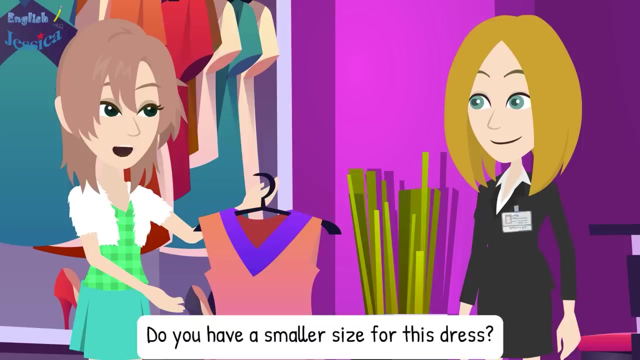 What would you like? I think I will try something new today. Can I try this on Sure? Excuse me, Excuse me, Hi, How can I help you? Do you have a smaller size for this dress? Yes, we have. Let me take it for you. Please wait a moment. 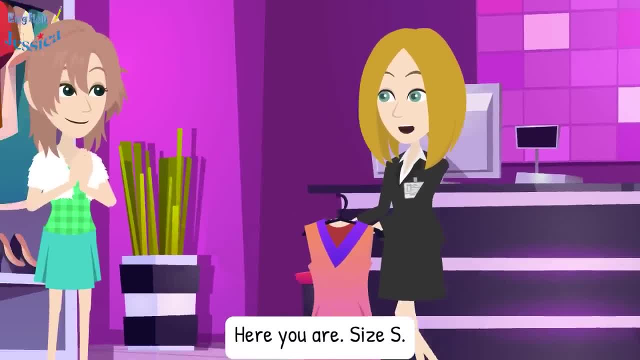 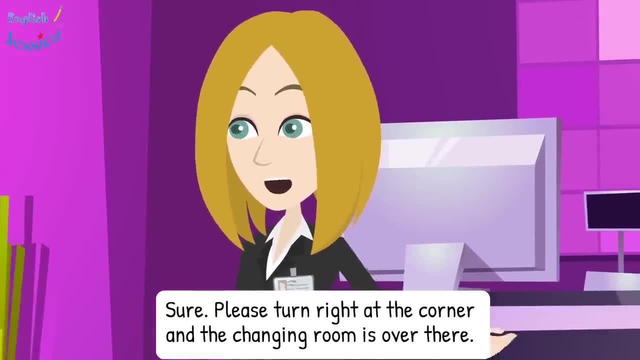 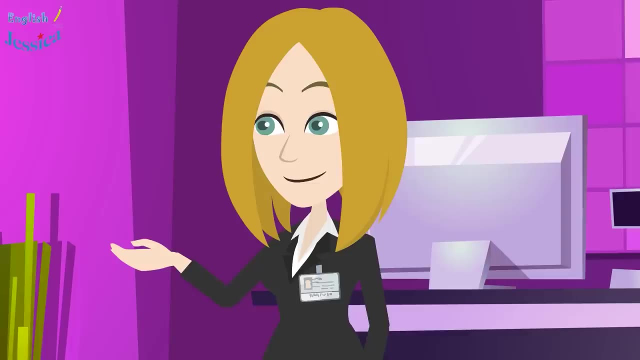 Okay, Here you are, Size, small. Can I try this on? Sure, Please turn right at the corner and the changing room is over there. Thank you, I think I will find more items to try all at once. Do you need me to help find anything? 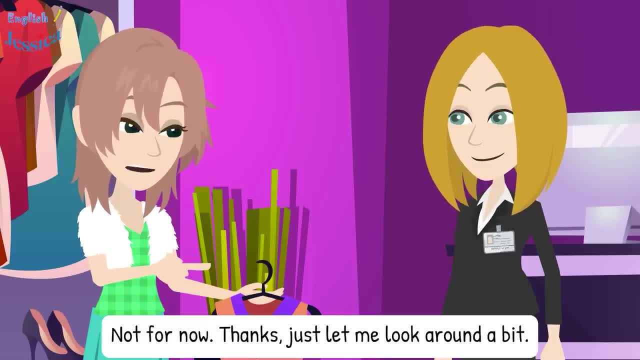 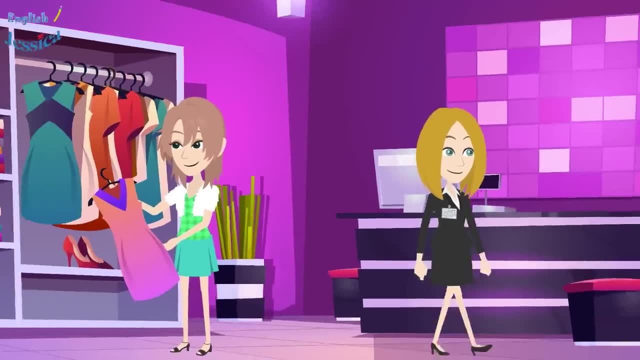 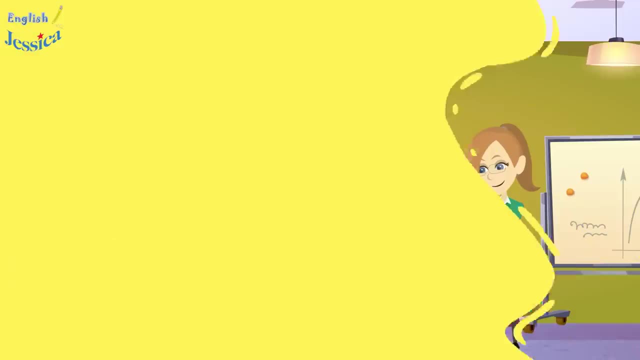 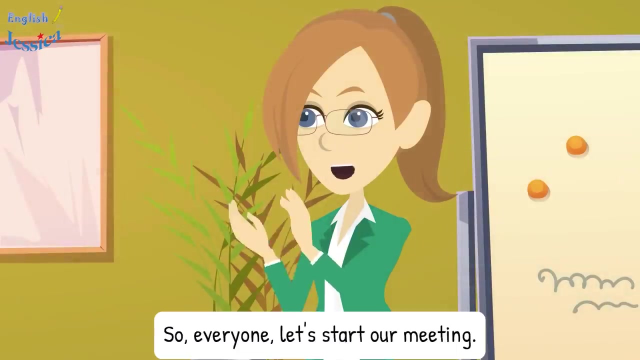 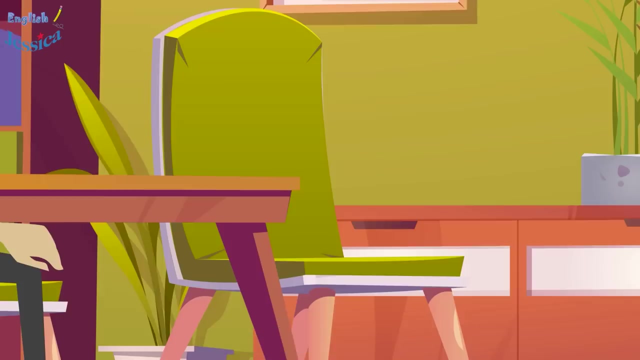 Not for now, thanks, Just let me look around a bit. Okay, take your time. Today I would like to outline our plans for the next project. So, everyone, let's start our meeting. Okay, Wait, where is Thomas? Thomas is sick today. He asked for a day off. 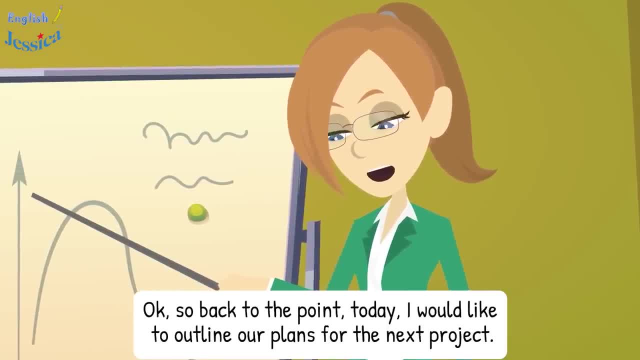 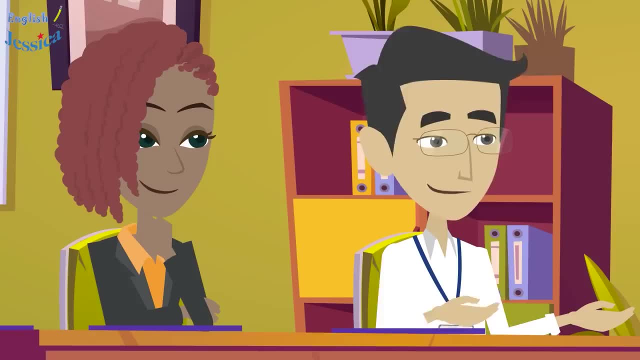 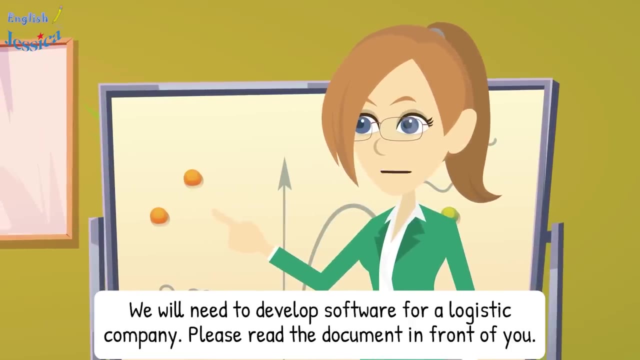 Okay, so back to the point. Today, I would like to outline our plans for the next project. When will it start? Next month? What is this project? We will need to develop software- Software for a logistic company. Please read the document in front of you. 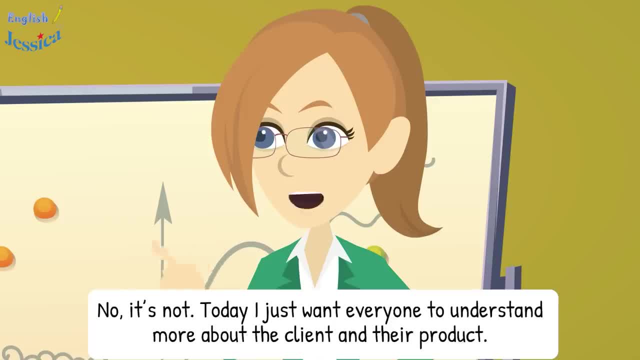 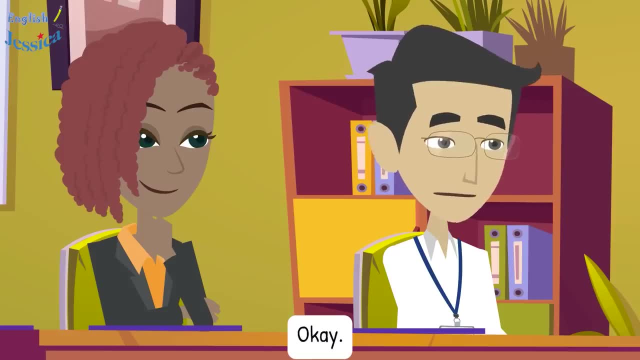 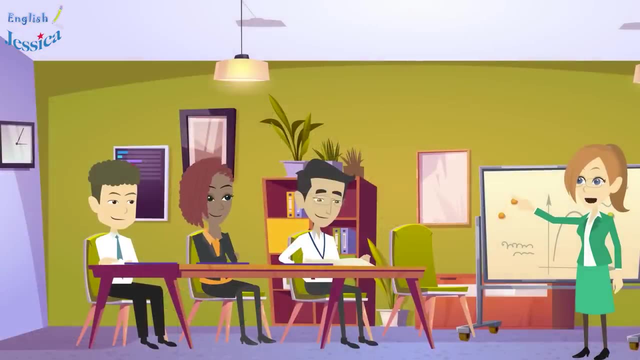 Is this a detailed description? No, it's not. Today, I just want everyone to understand more about the client and the product. Okay, Now please read it first before we discuss more about this project. Can you please gift wrap it for me? 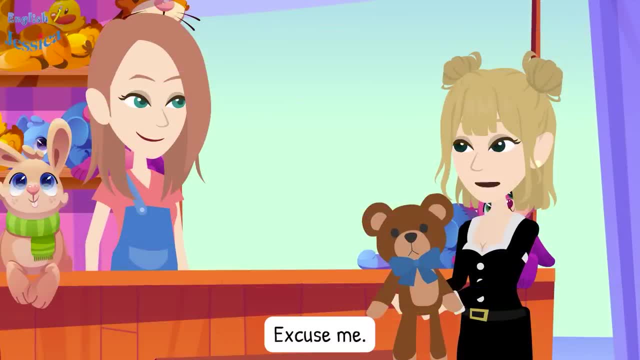 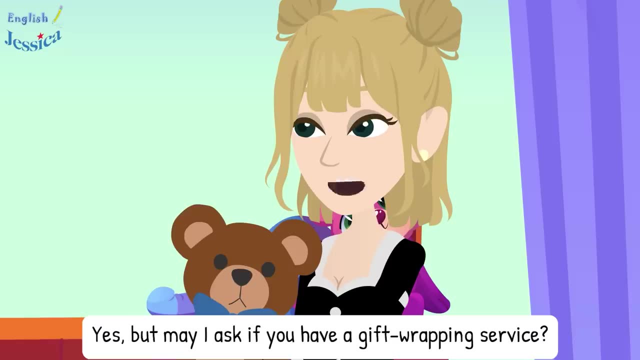 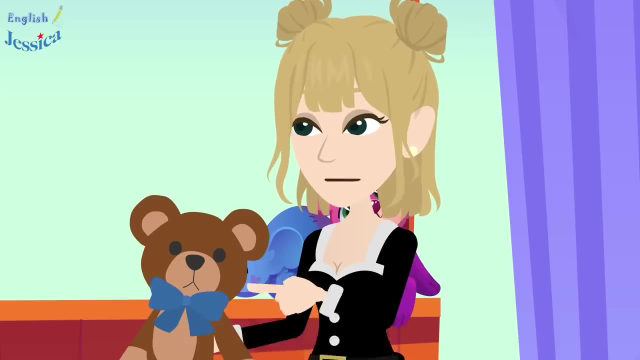 Yes, ma'am, Excuse me. Hello, do you want to check out? Yes, but may I ask if you have a gift wrapping service? Yes, we have. What do you need to wrap This teddy bear? Okay, it costs $3 more for gift wrapping, Is it okay for you? 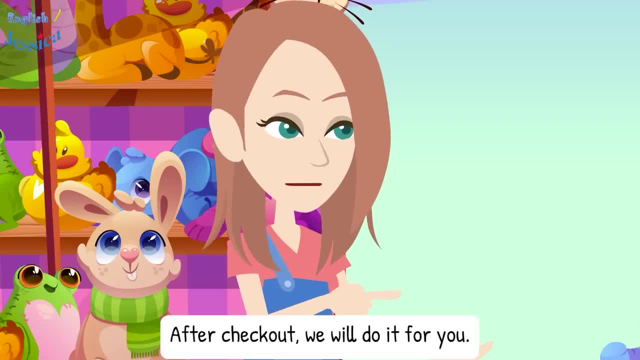 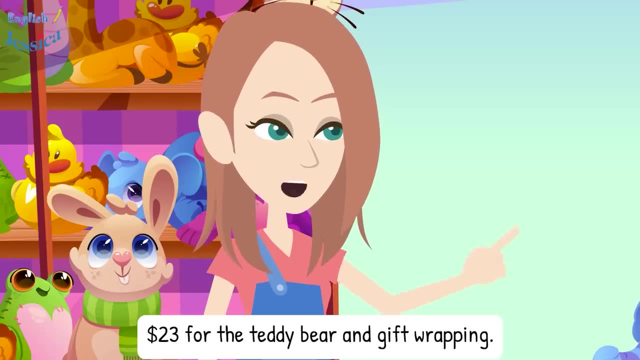 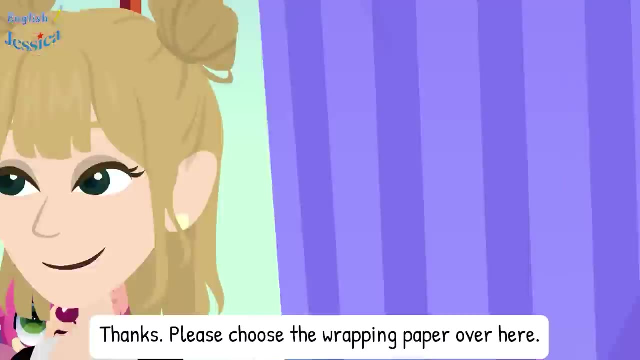 Yes, After checkout, we will do it for you. Okay, How much is it in total? $23 for the teddy bear and gift wrapping. Okay, here you are. Thanks, Please choose the wrapping paper over here, This one. 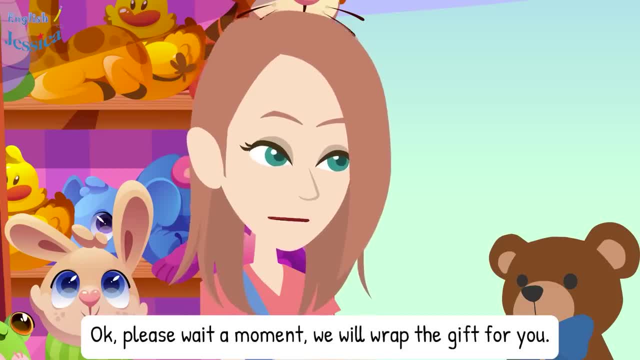 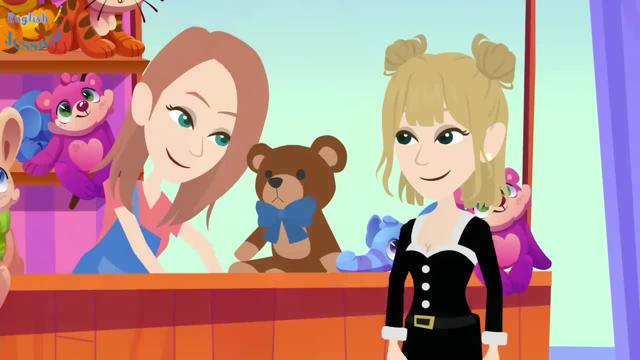 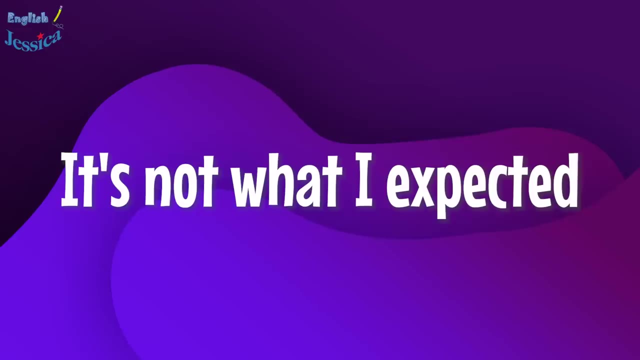 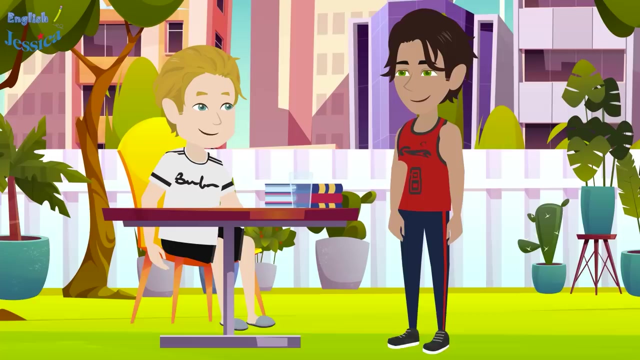 Okay, please wait a moment. We will wrap the gift for you. Okay, Thank you, You are welcome. You are welcome. It's not what I expected, Joe. how is your thesis going? It's good. I'm writing a conclusion, Nearly finished. 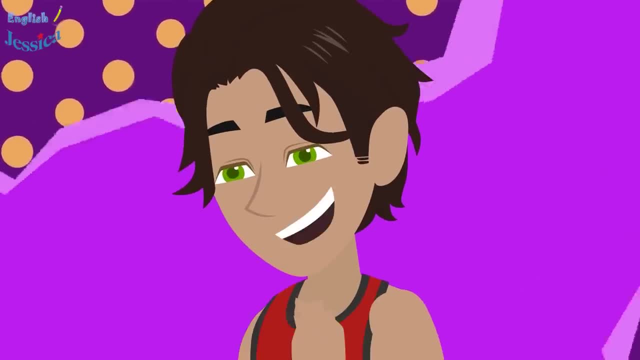 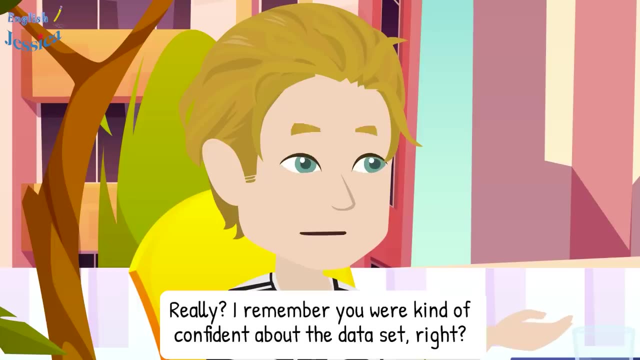 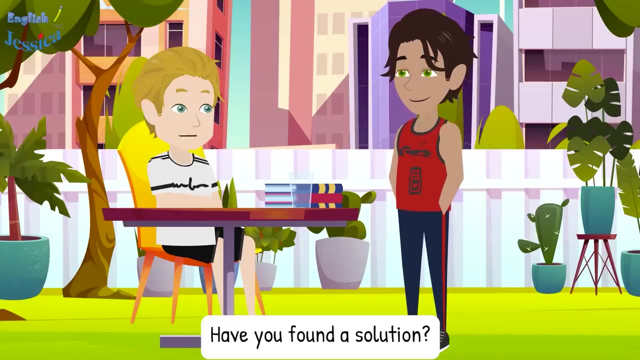 Wow, impressive, You're so quick. How about you? I have a problem with the data Really. I remember you were kind of confident about the data set right. Yeah, it's not what I expected. Have you found a solution? 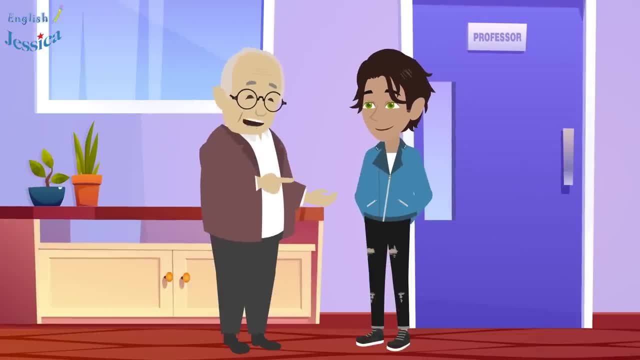 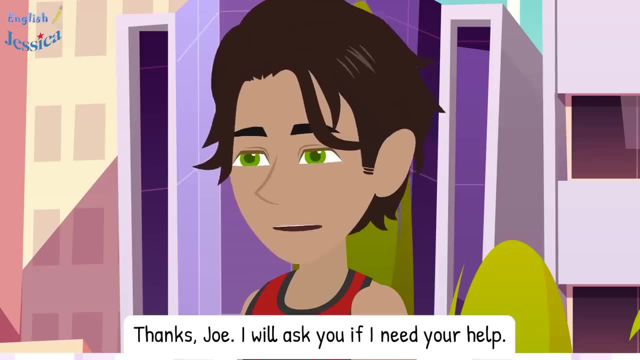 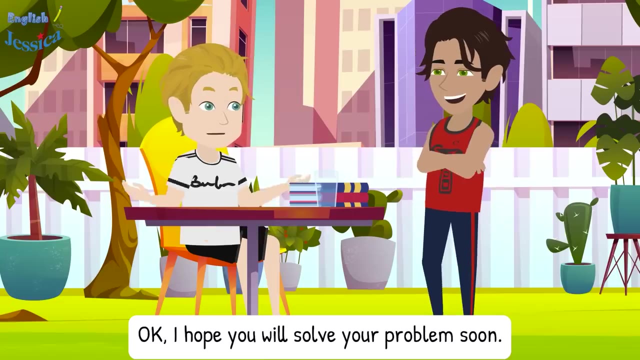 I'm going to consult my professor this afternoon. Is there anything I can help? My one will be finished soon. anyway, Thanks, Joe, I will ask you if I need your help. Okay, I hope you will solve your problem soon. Looking forward to seeing you soon. 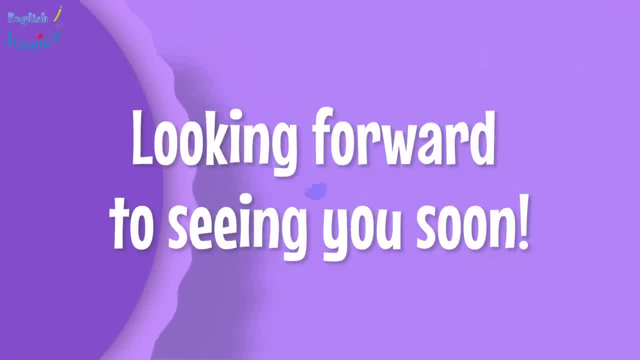 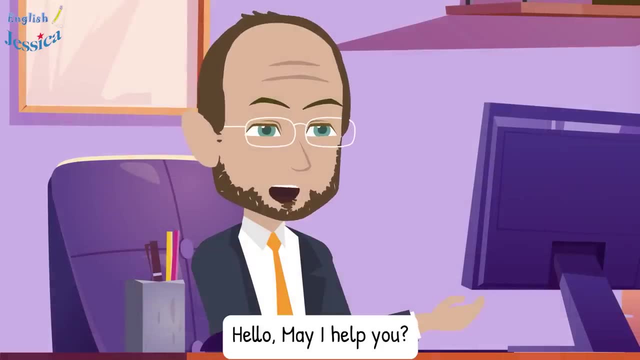 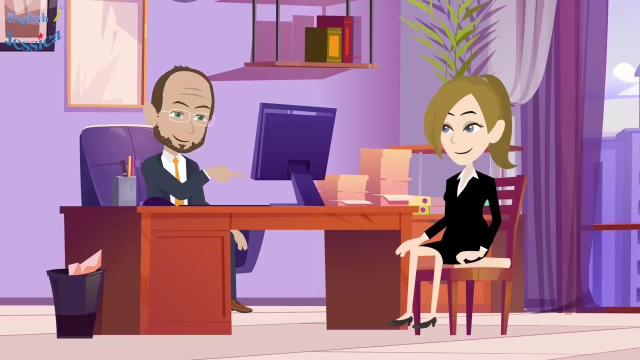 Looking forward to seeing you soon. Hello, may I help you? Hi, I want to find a job. Do you have any vacancies? Well, first of all, do you have a CV? Yes, I have. Please take a look. 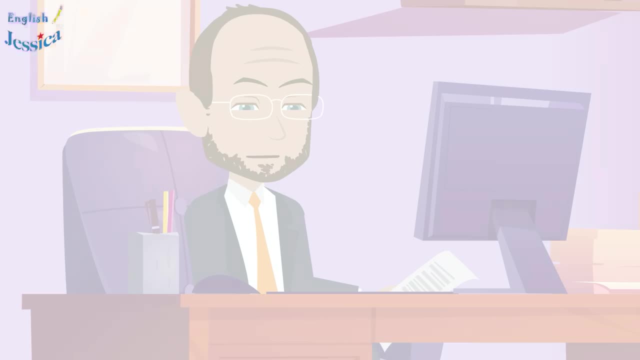 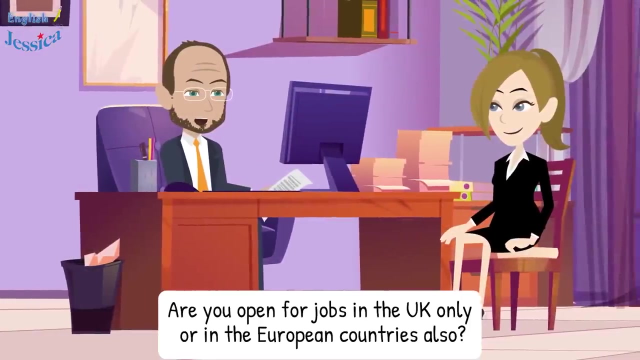 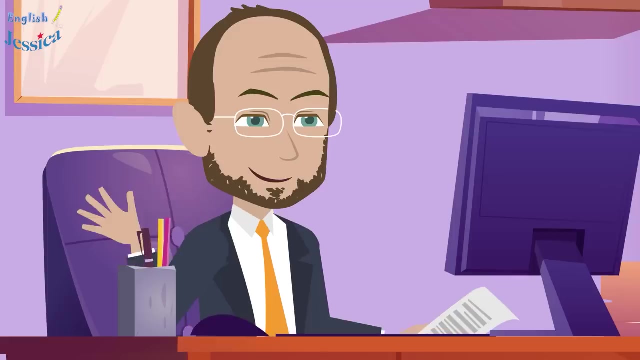 In what field do you want to work? I want to work in IT front-end development. Are you open for jobs in the UK only or in the European countries also? I am open to jobs in the UK. Okay, Do you have a preference for the city you want to work in? 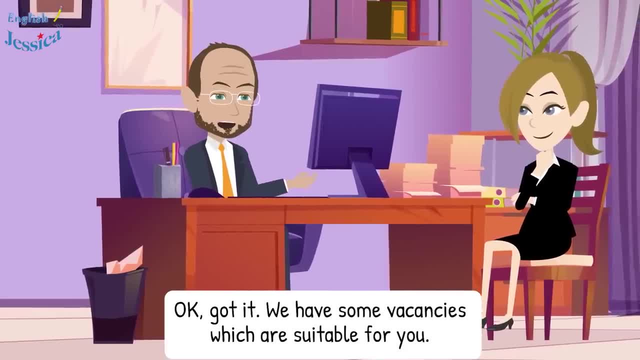 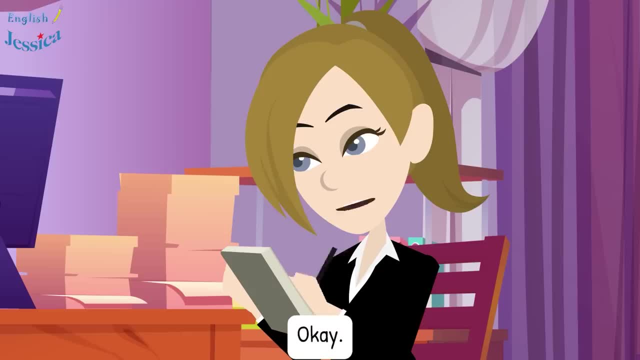 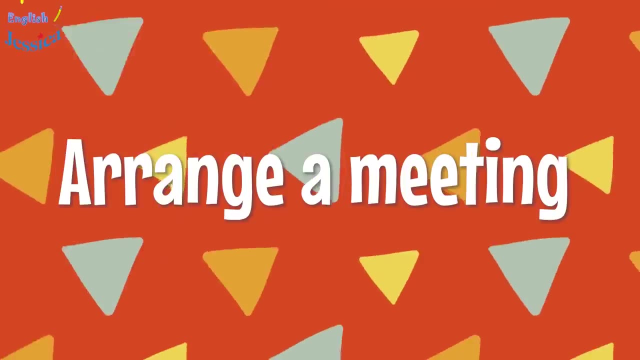 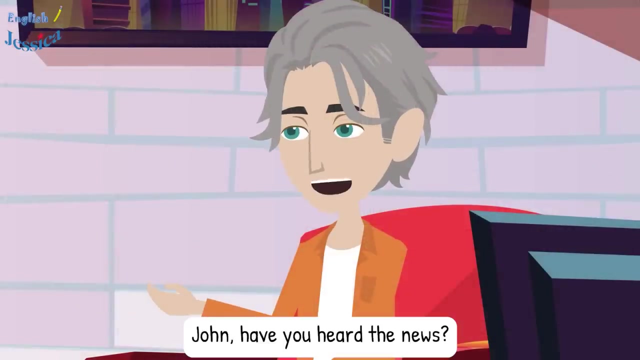 I like London. Okay, got it. We have some vacancies which are suitable for you. Please choose the ones you want to apply. Okay, Arrange a meeting, John. have you heard the news? What news? Tony will come back next week. 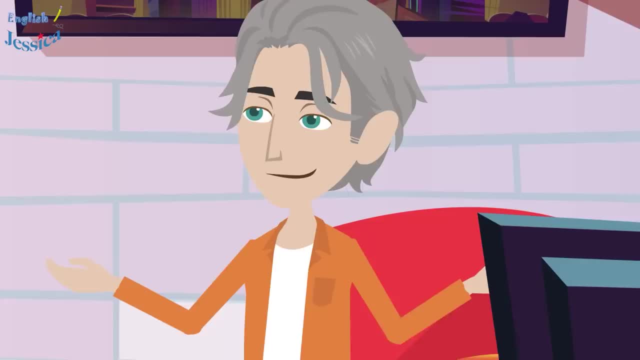 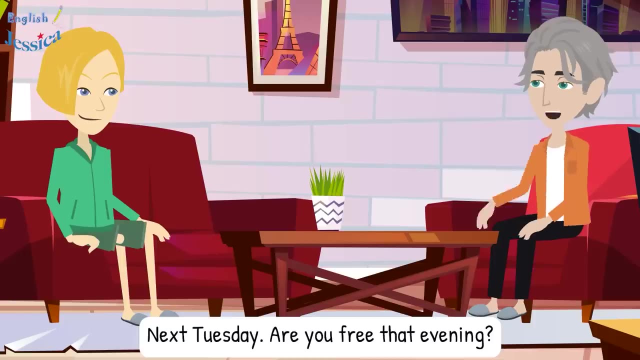 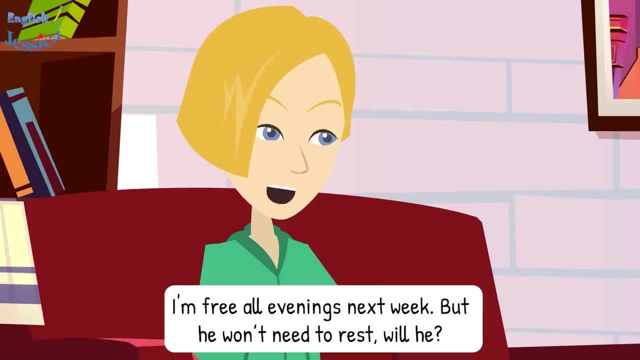 Really, Do you know how long he will stay? I'm not sure, but he told me he wanted to meet up. Sure, When will he be here Next Tuesday? Are you free that evening? I'm free all evenings next week, but he won't need to rest, will he? 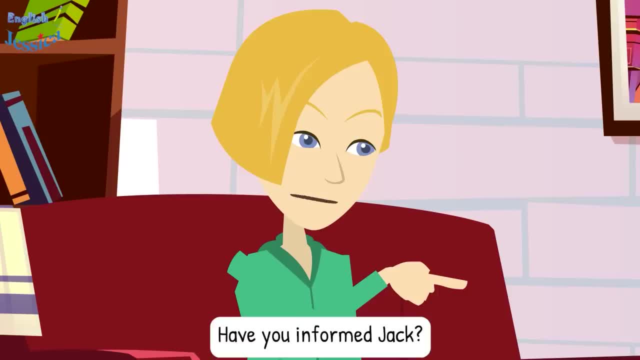 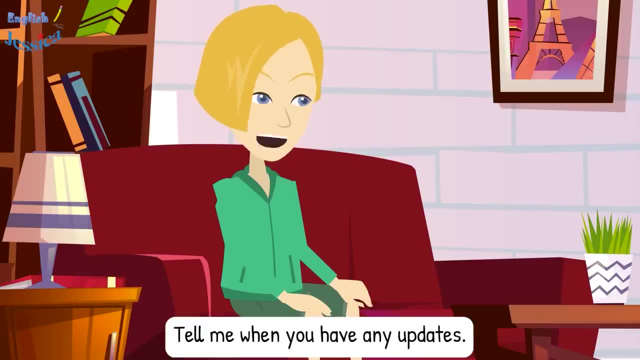 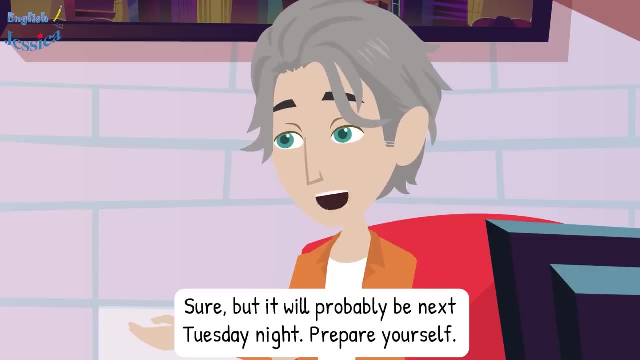 I'm not sure. I will ask him again. Have you informed Jack? Not yet. I will call Jack now. Okay, Tell me when you have any updates. Sure, but it will probably be next Tuesday night. Prepare yourself, Got it? 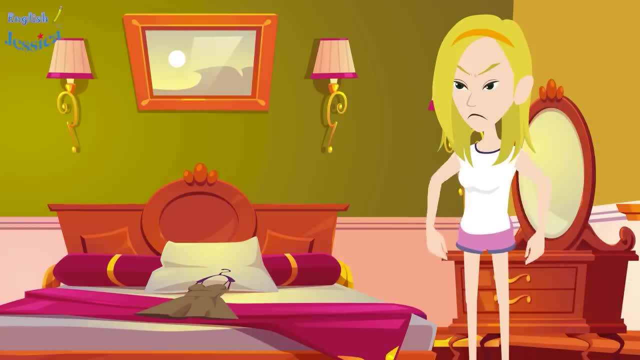 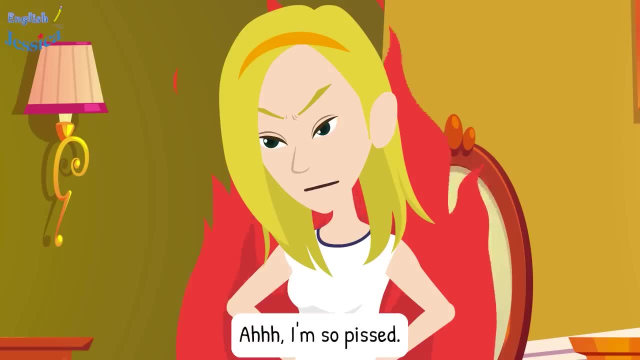 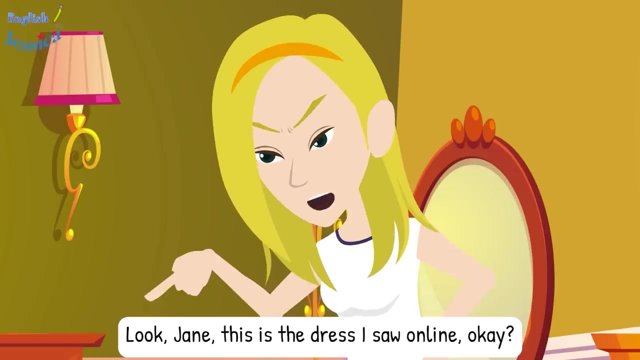 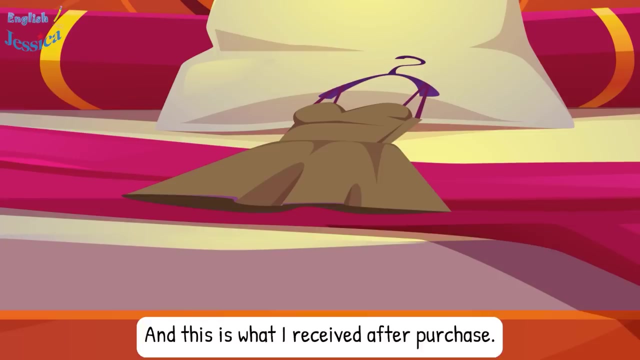 Being angry? What's wrong, Sophia? I'm so pissed. Why are you so angry? Look, Jane, This is the dress I saw online. okay, Yeah, And this is what I received after purchase. Oh my gosh, Is it the same thing? 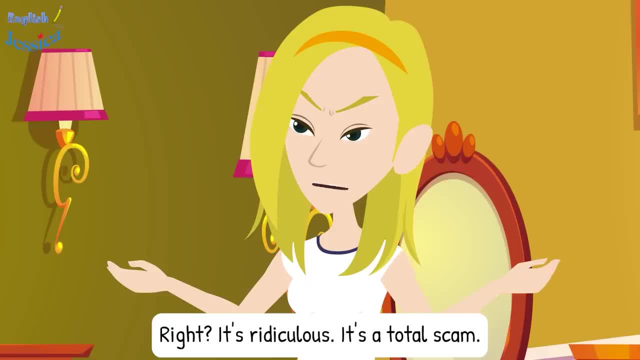 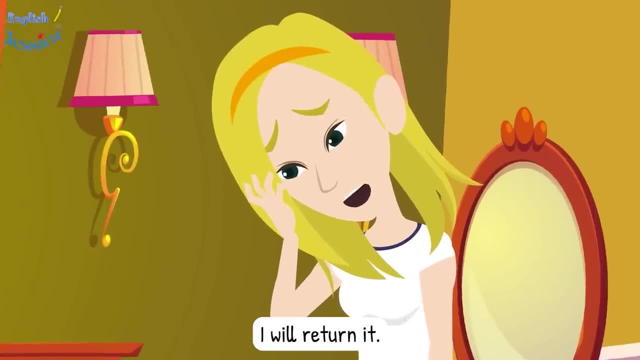 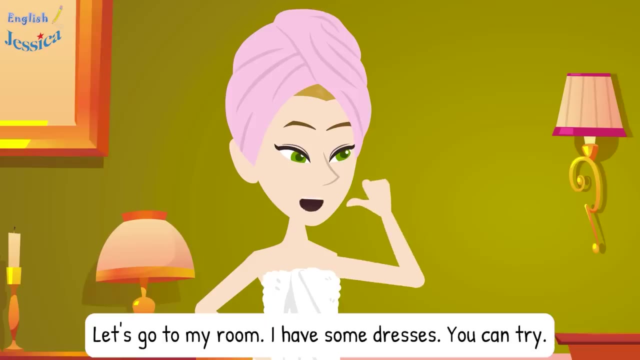 Right, It's ridiculous. It's a total scam. I can feel you. I would be so angry too if I were you. I will return it, But I bought it for this evening party. What can I do now? Let's go to my room. I have some dresses you can try. 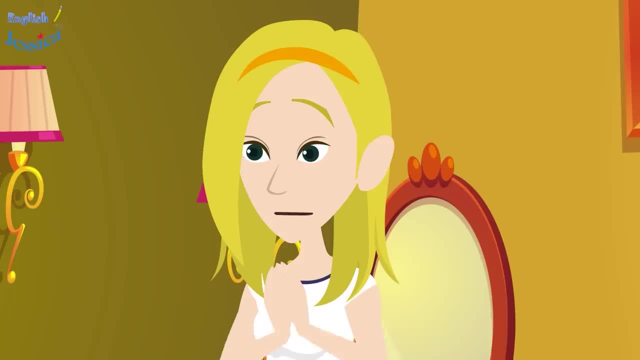 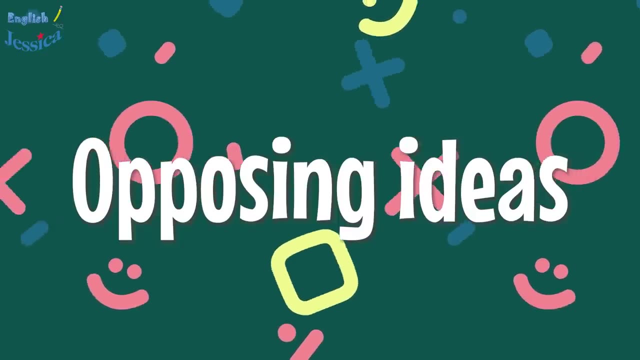 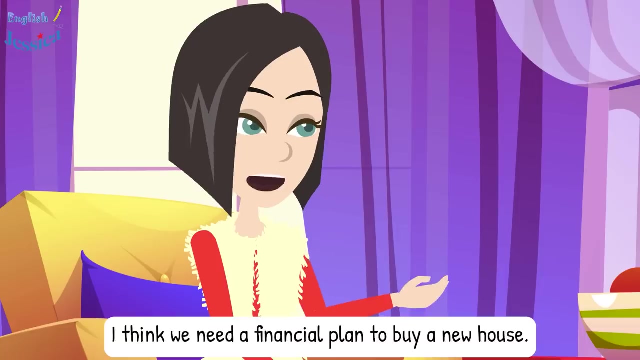 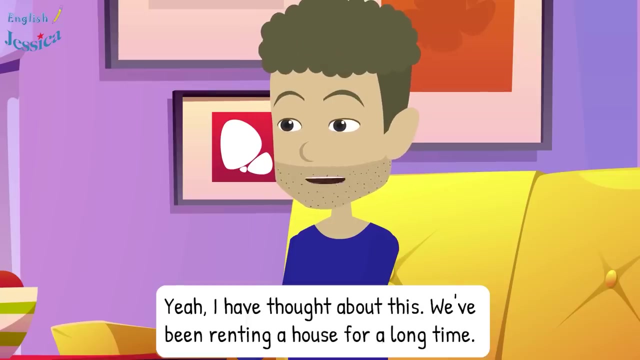 Oh, thank you so much, Jane. Oh, thank you so much, Jane. Opposing ideas: Honey, I think we need a financial plan to buy a new house. Yeah, I have thought about this. We've been renting a house for a long time. 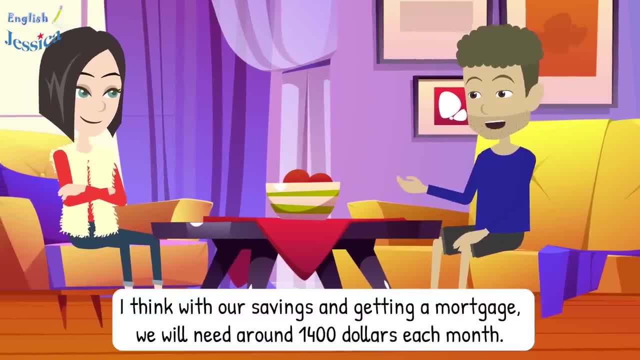 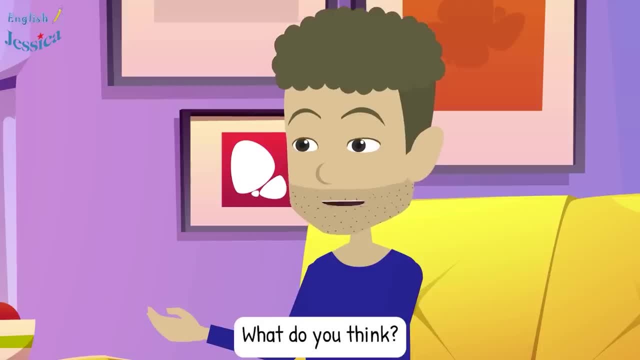 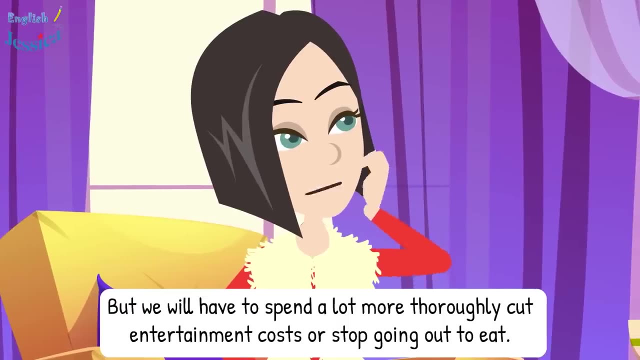 So what is the plan? I think, with our savings and getting a mortgage, we will need around $1,400 each month. What do you think? That's okay, But we will have to spend a lot more thoroughly, cut entertainment costs or stop going out to eat. Let's eat at home from now on. 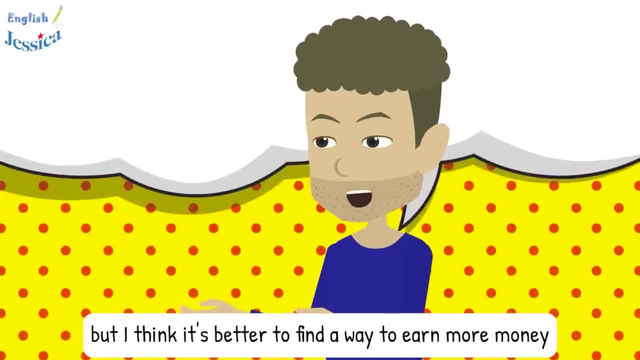 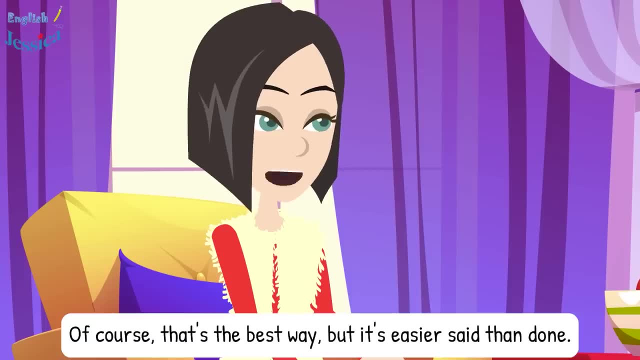 I understand what you mean, But I think it's better to find a way to earn more money instead of having to budget on everything like that. Of course, that's the best way, But it's easier said than done. Do you have any plans to earn more? 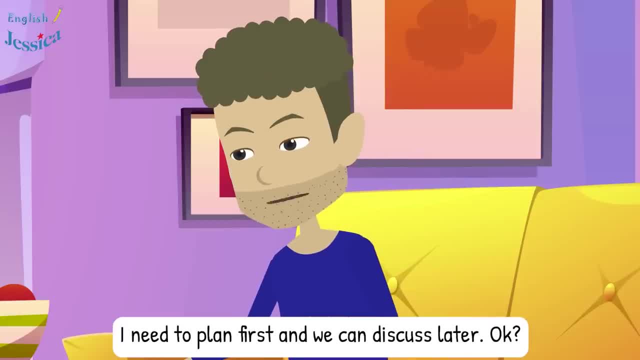 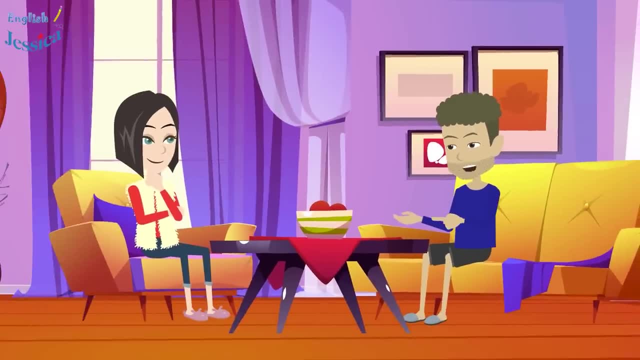 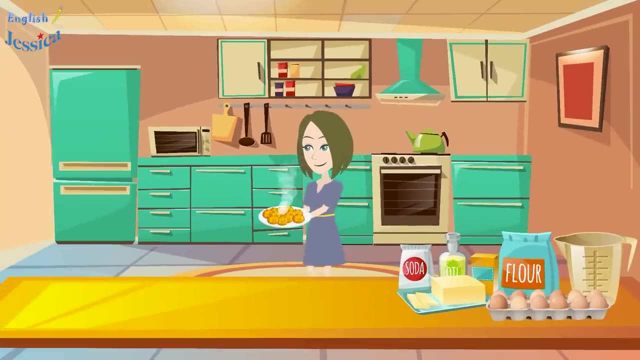 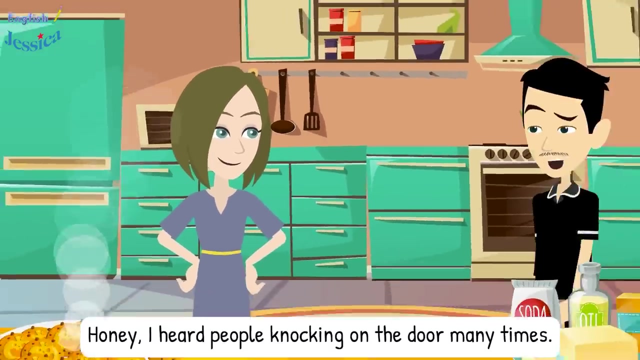 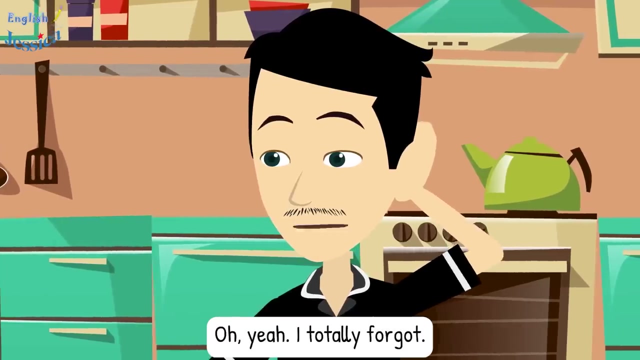 I need to plan first and we can discuss later. okay, Okay, Five senses, Three senses, Two senses, One senses, Two senses. Honey, I heard people knocking on the door many times. Those were the kids playing trick or treat. Oh yeah, I totally forgot. I saw many kids with cute customs on the way home today. 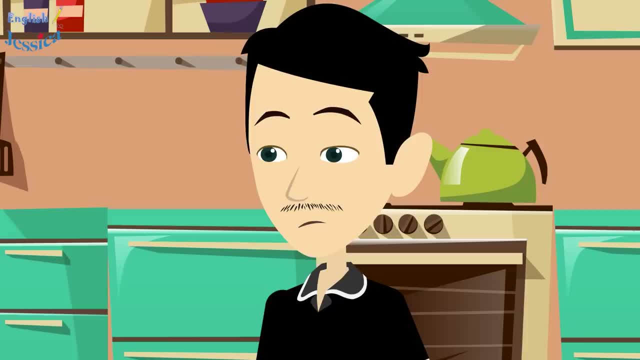 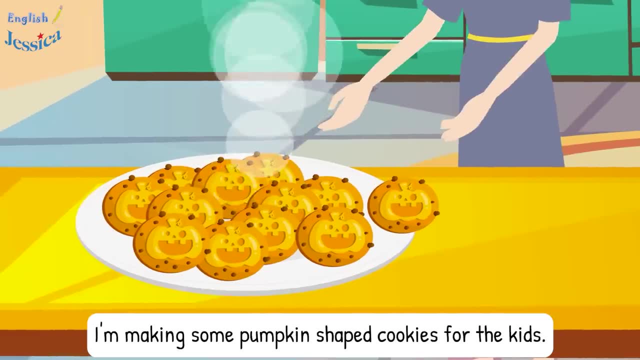 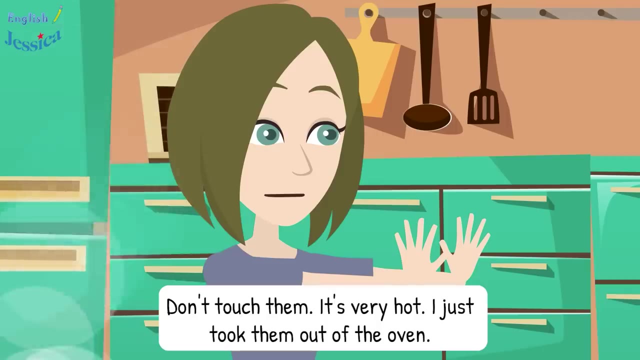 There was even a dinosaur coming over. Really, Oh, what are you doing? It smells so good. It smells so good. I'm baking some pumpkin-shaped cookies for the kids. Let me try one. Don't touch them, It's very hot. I just took them out of the oven. 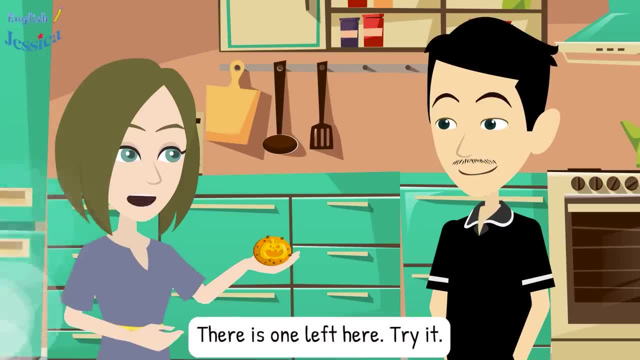 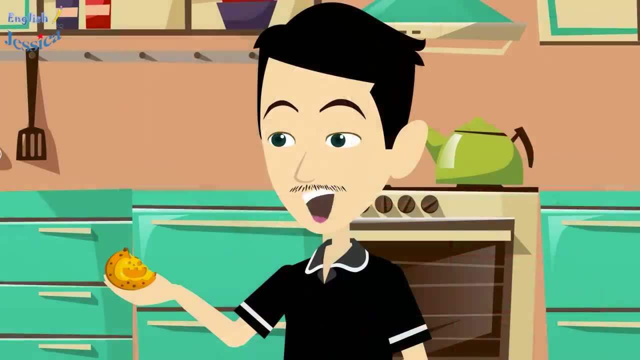 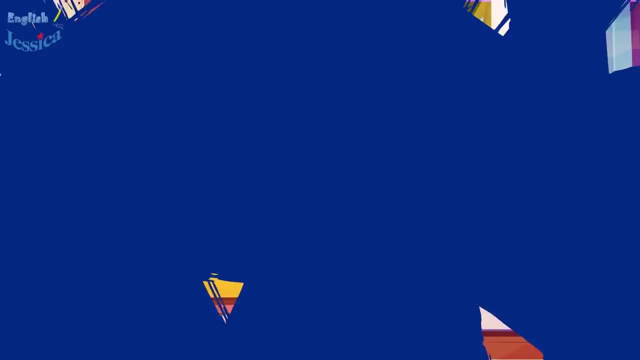 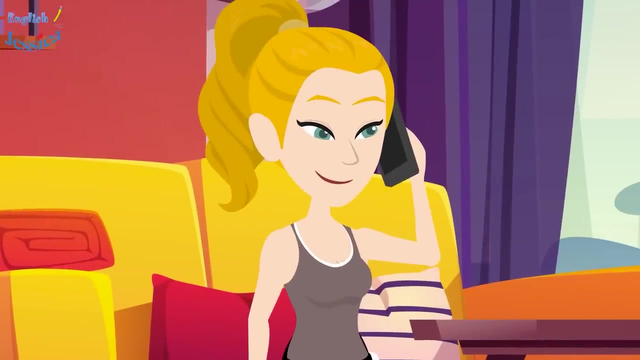 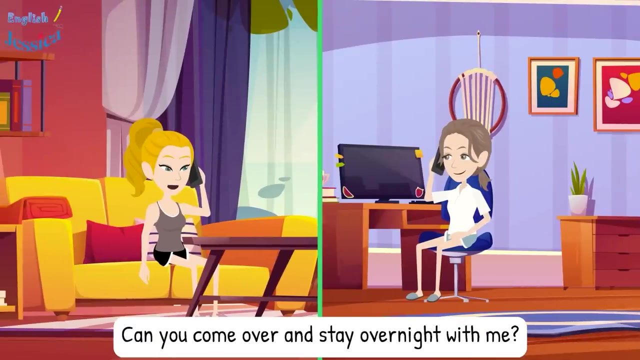 Fine, There is one left here, Try it. Oh, it tastes really delicious. Thanks, Phone call. Hey Laura Girl, what's up? My parents are not at home tonight. Can you come over and stay overnight with me? 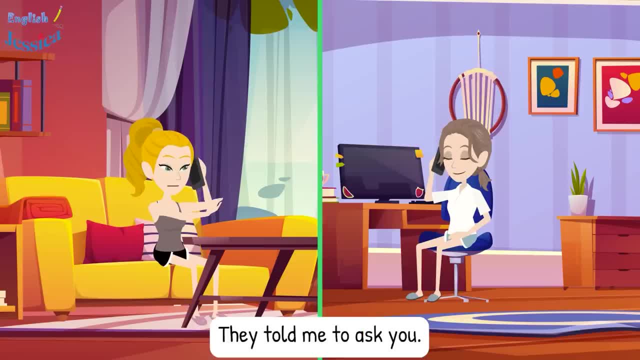 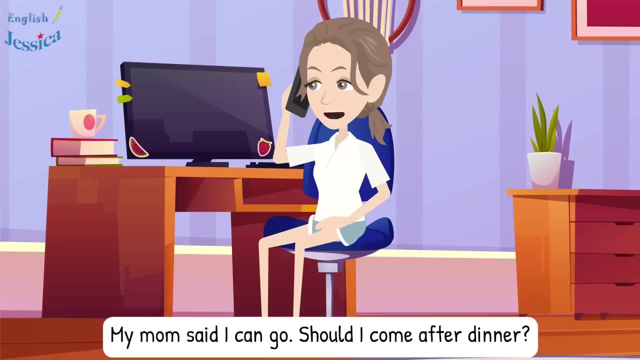 Sure, Have you asked your parents? They told me to ask you. Okay, Let me ask my mom first, then I call you back. okay, Sure, Hey, how was it? My mom said I can go. Should I come after dinner? 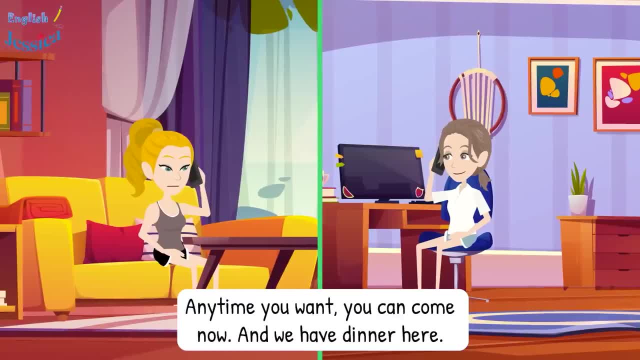 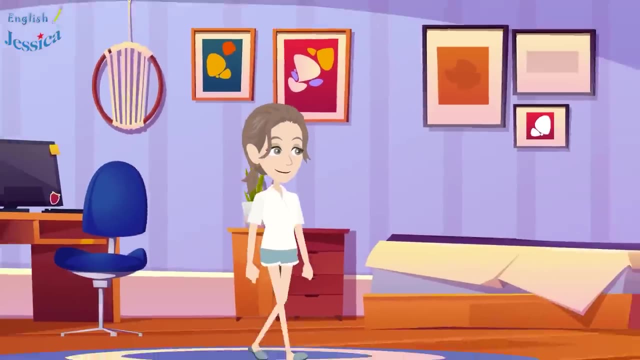 Anytime you want. You can come now and we have dinner here. Okay, Let me prepare. I will be there in 30 minutes. Okay, Bye, Bye. Good morning, How can I help you? Hi, I received a notice that my package has arrived at the post office. Can I get it now? 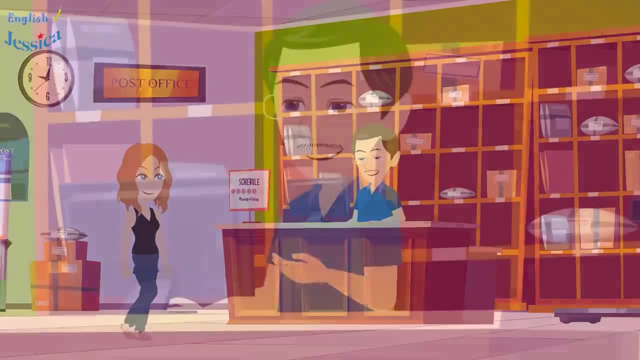 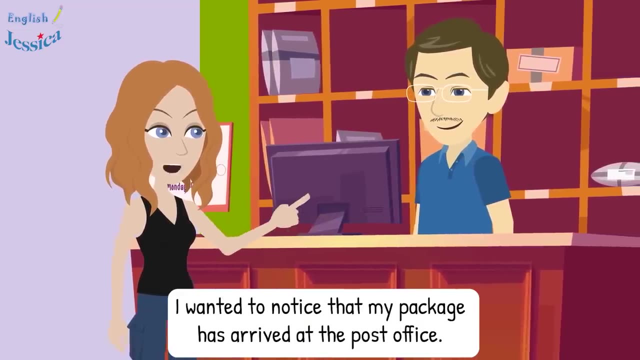 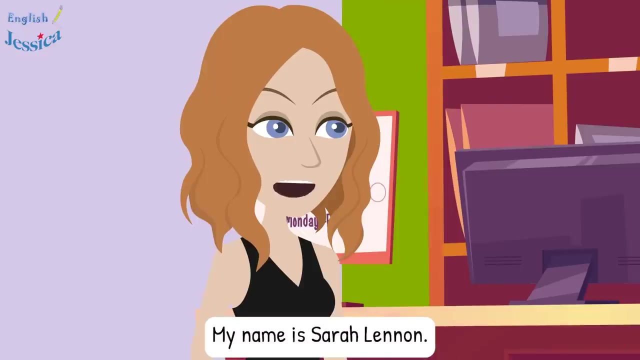 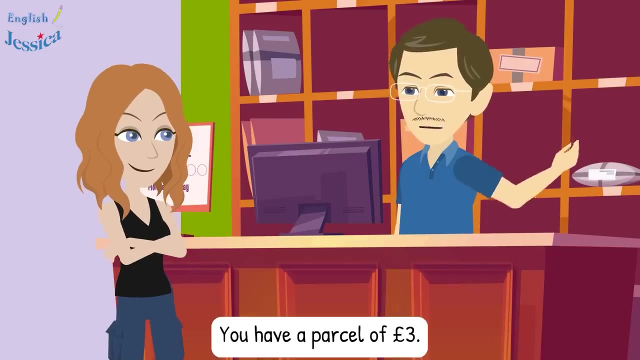 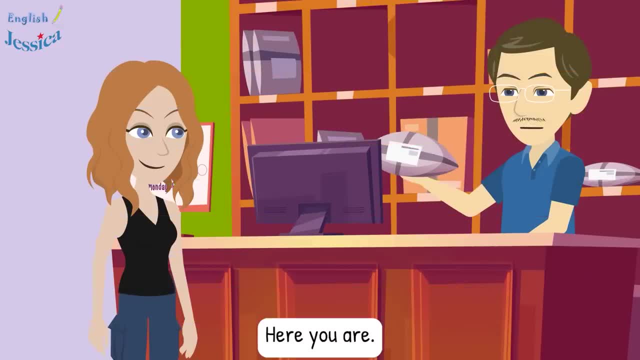 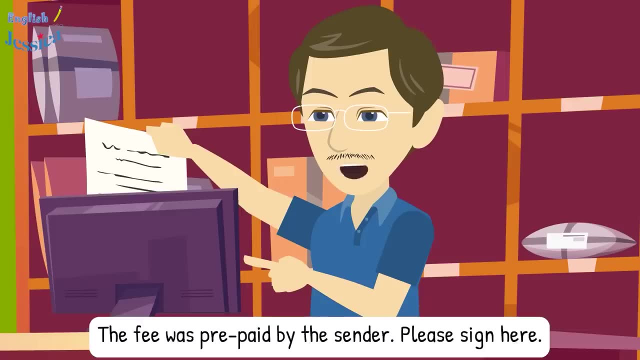 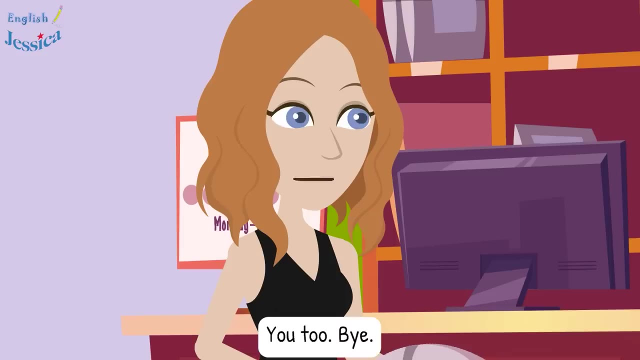 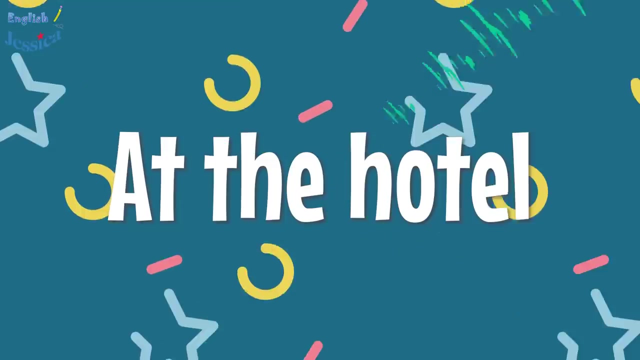 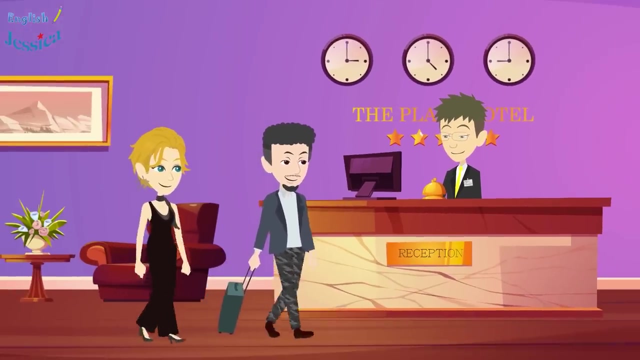 Okay, Thanks, Here you are. How much is the shipping fee? The fee was prepaid by the sender. Please sign here. Okay, Thank you. Have a nice day You too. Bye, Good afternoon. Welcome to the Plaza Hotel. How can I help you, sir? 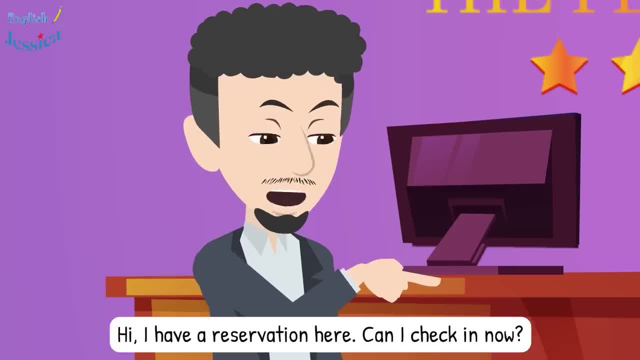 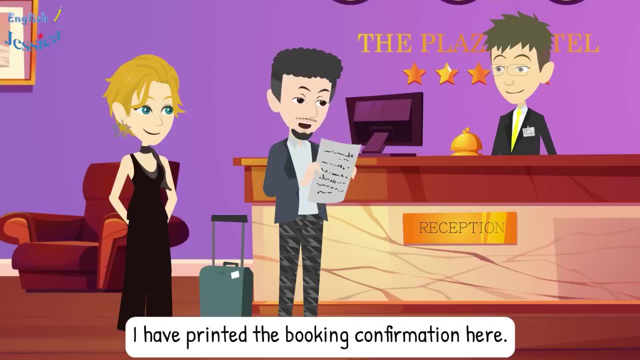 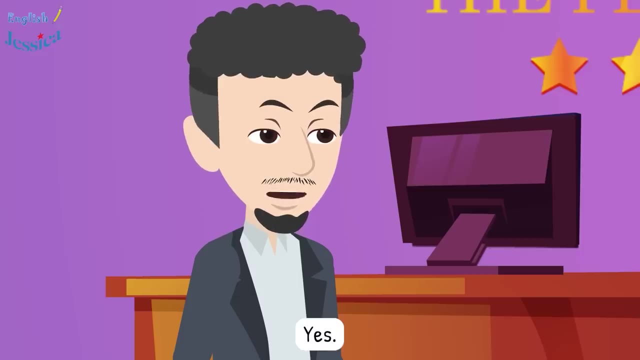 Hi, I have a reservation here. Can I check in now? Sure, sir, May I have the booking number and your name please? I have printed the booking confirmation here. Please check. Let me check. Yes, Okay, I got it. Could I have your identity cards please? 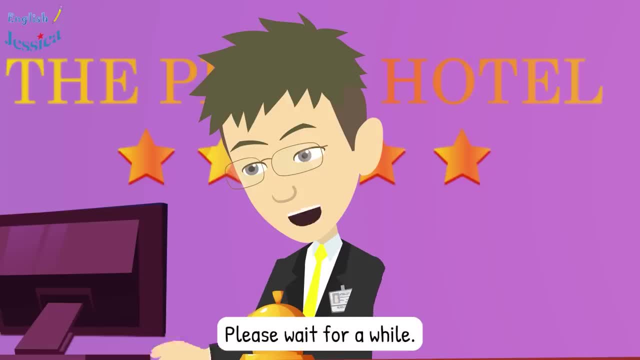 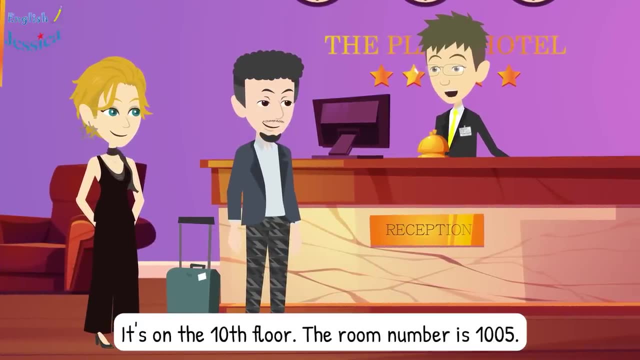 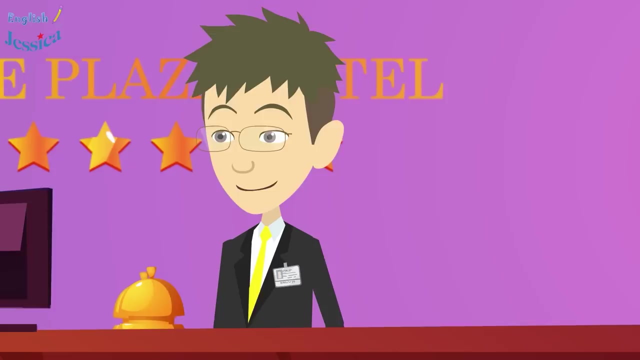 Yes, Here you are. Please wait for a while. Okay, Your room is ready, sir. It's on the 10th floor. The room number is 1005.. Here are your ID cards and room key cards. Great, Our bellman will help you to bring your luggage and take you to the room. 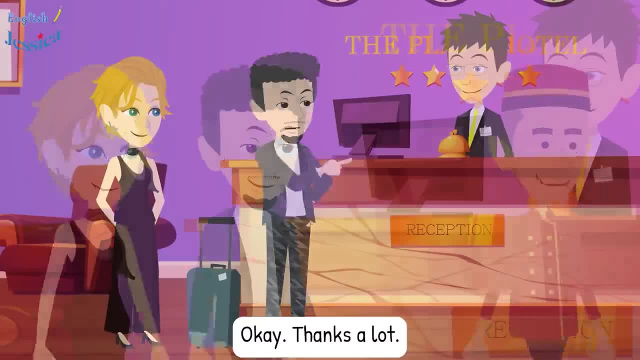 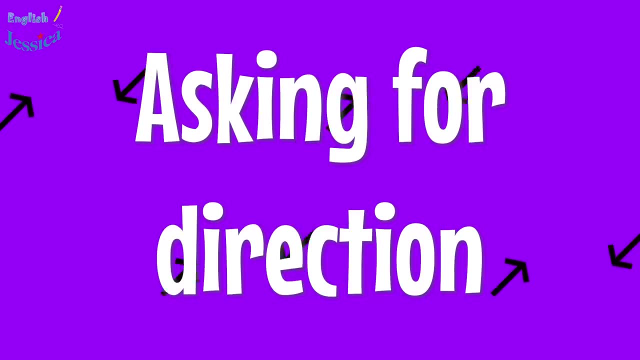 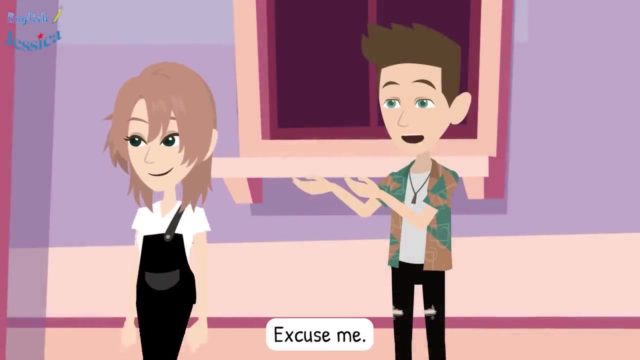 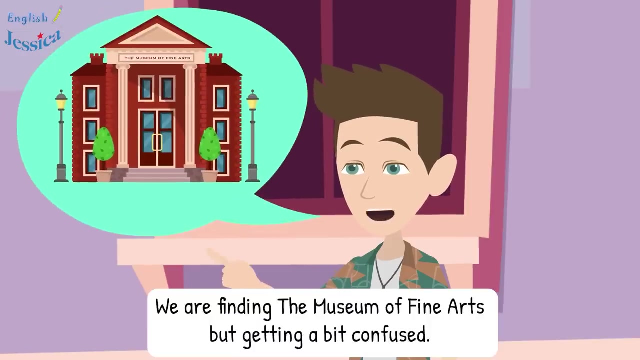 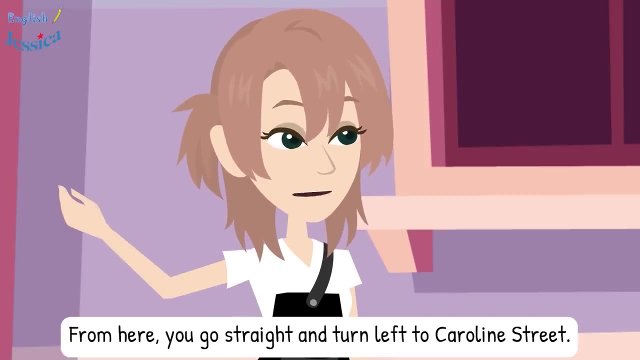 Okay, Thanks a lot Asking for directions. Excuse me, Hi, How can I help you? We are finding the Museum of Fine Arts, but getting a bit confused. Could you show me the way to get there, please? Ah sure, From here you go straight and turn left to Caroline Street. 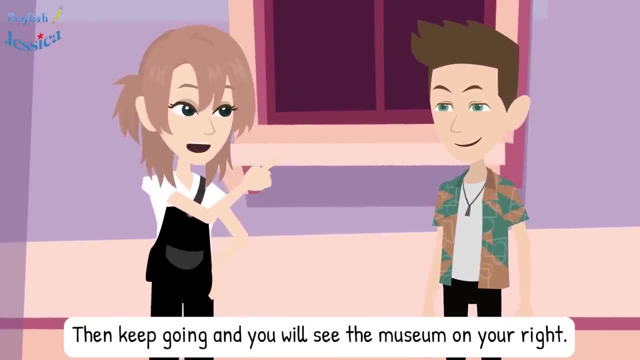 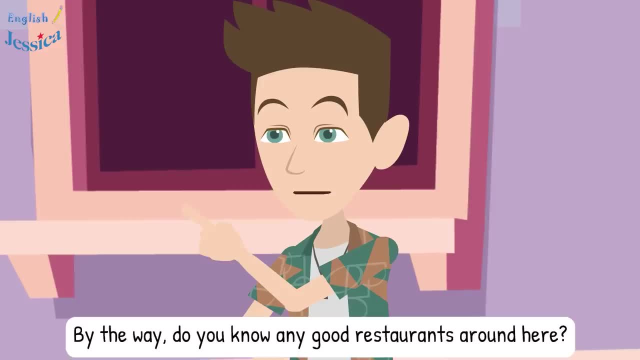 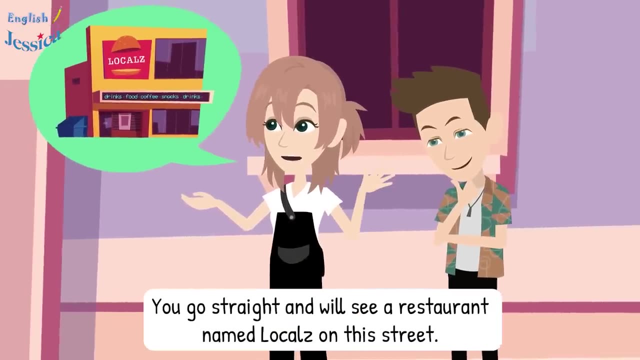 Go ahead and turn right to Bin Street, Then keep going and you will see the museum on your right. Thanks a lot for your help. Not at all, By the way. do you know any good restaurants around here? Ah yeah, You go straight and you will see a restaurant named Locales on the street. 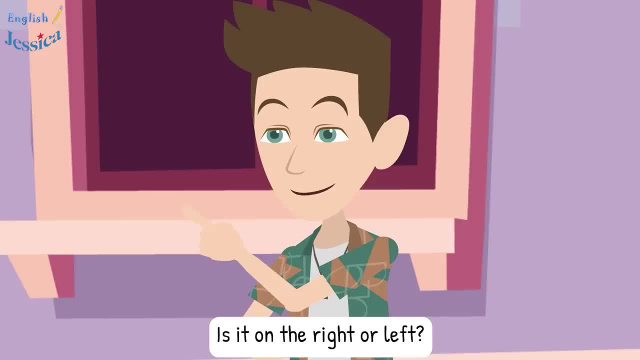 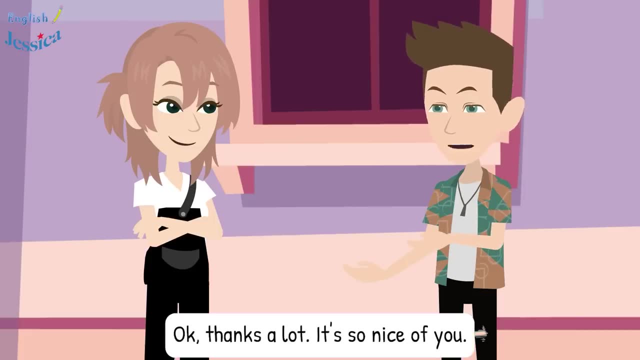 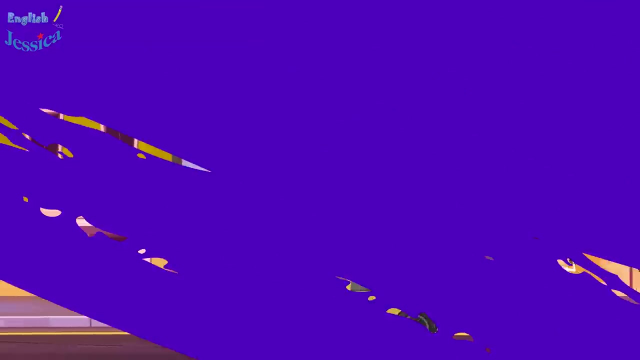 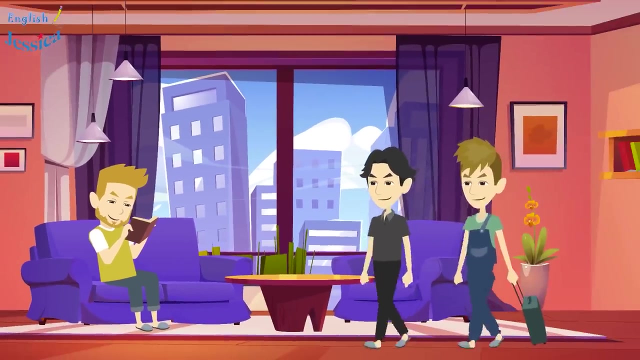 It's a small one, but the food is really delicious. Is it on the right or left? On your right, Okay, Thanks a lot. It's so nice of you. You're welcome. Self-introduction. Hey, Tom, This is Bob, my cousin. He would stay with me for a few days. 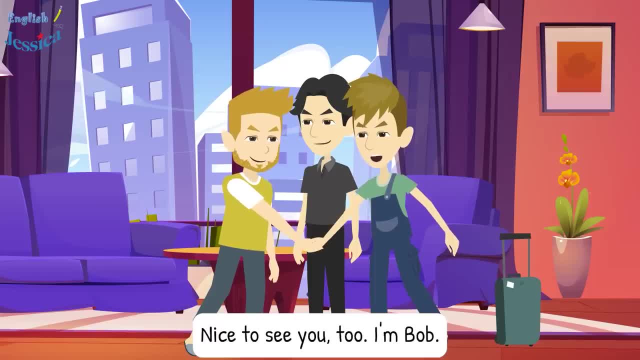 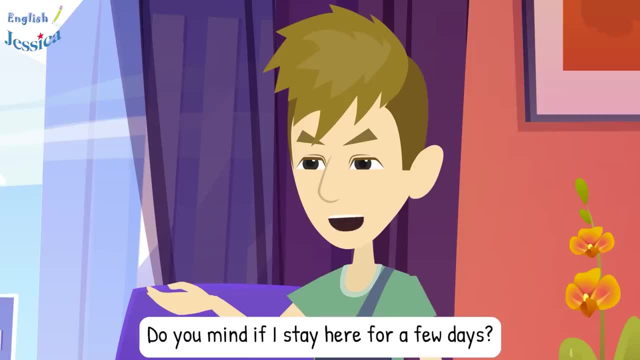 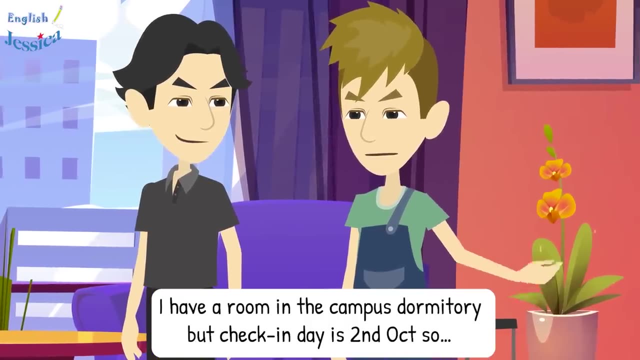 Hi Bob. Nice to see you. Nice to see you too. I'm Bob. I'm a freshman at Boston University. Do you mind if I stay here for a few days? No problem, I have a room in the campus dormitory, but check-in day is 2nd of October, so…. 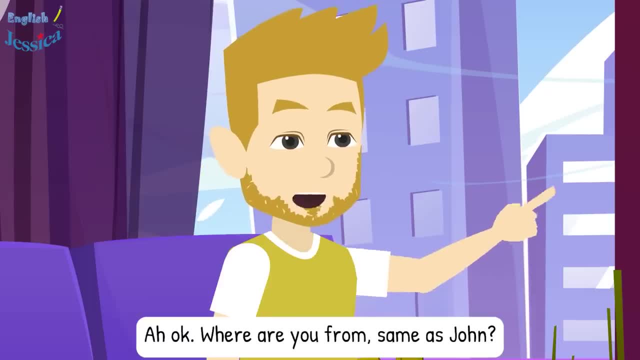 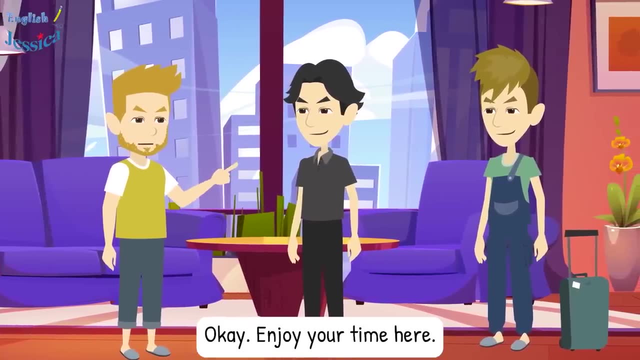 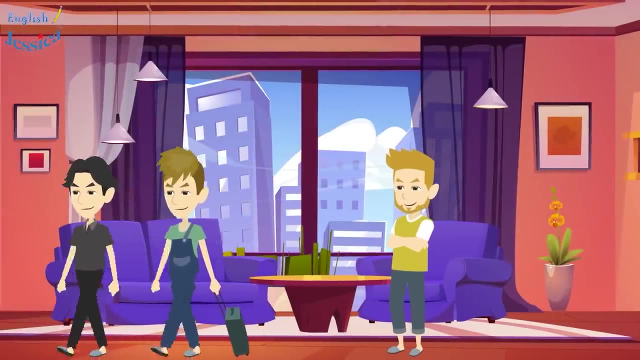 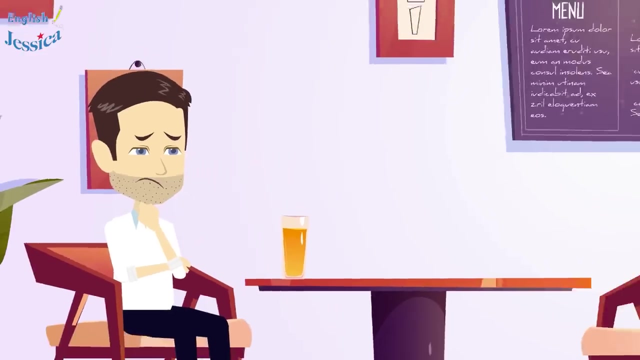 Ah, okay, Where are you from, Same as John? Yes, I'm from Bristol. Okay, Enjoy your time here. We can take him around the area this afternoon. Great Marriage- What are you thinking, man? Hi, Jake, I'm thinking about how to celebrate our wedding anniversary. 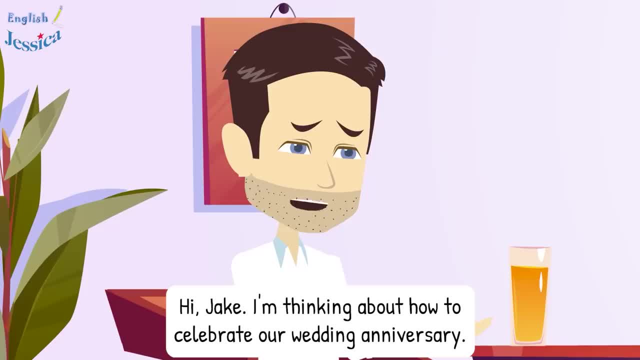 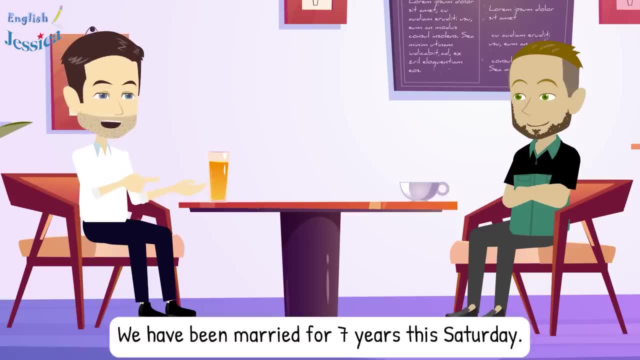 Oh really, How long have you and Alisa been married? We've been married for 7 years This Saturday. Wow, that's long, though. What's the tip? There's no tip. Just spending time together and helping each other. 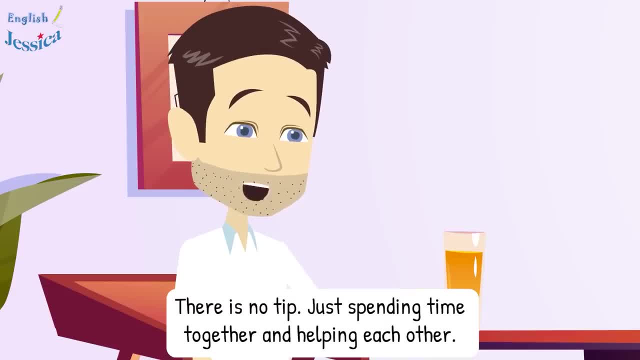 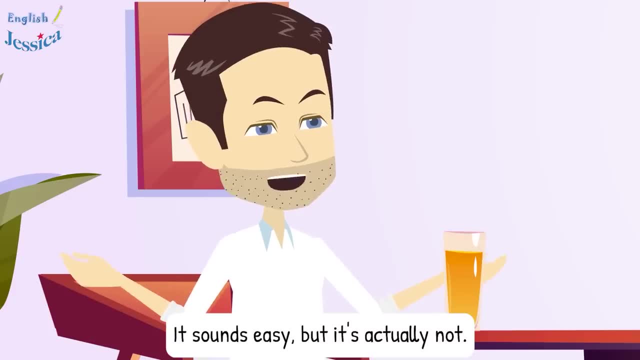 Okay, I'll see you tomorrow, Spending time together and helping each other. That's it. It sounds kind of easy, though It sounds easy, but it's actually not. You're right, Sometimes we are too busy to care for our beloved. 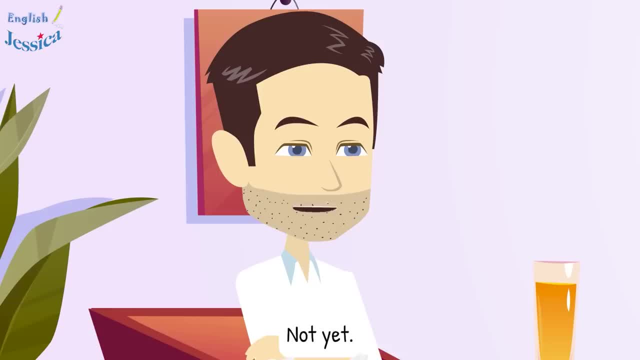 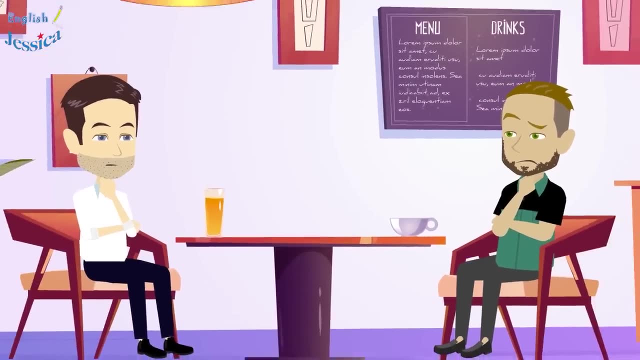 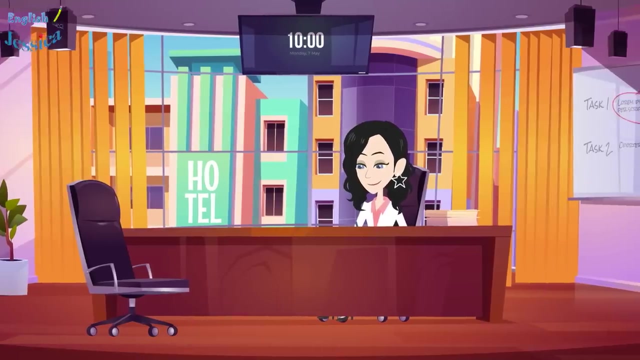 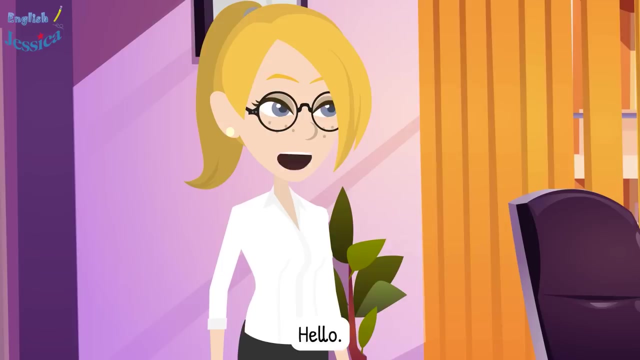 So have you got the idea yet? Not yet? Okay, I will let you focus A few weeks later. Job Interview: Come in please. Hello, Hello. I'm Sarah. I'm a marketing manager. Please take a seat. 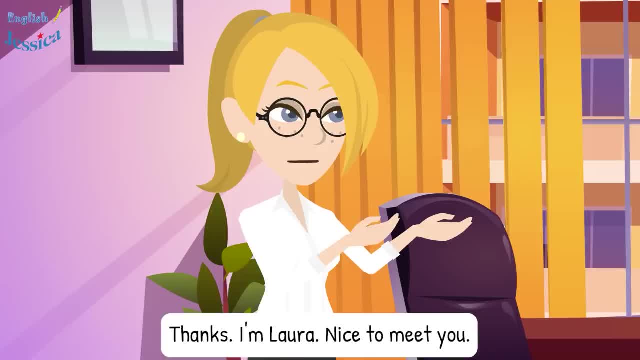 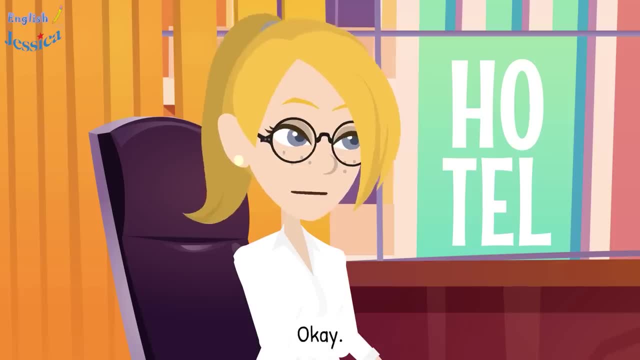 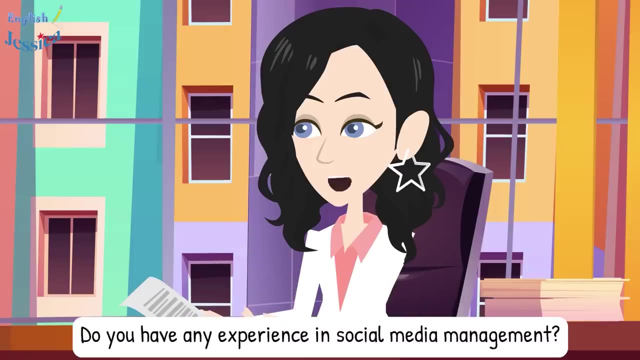 Thanks, I'm Lauren, Nice to meet you. Okay. Today I am your interviewer. Let's start Okay. today I'm your interviewer. Let's start Okay. I see that you have worked in a marketing position before. Do you have any experience in social media management? 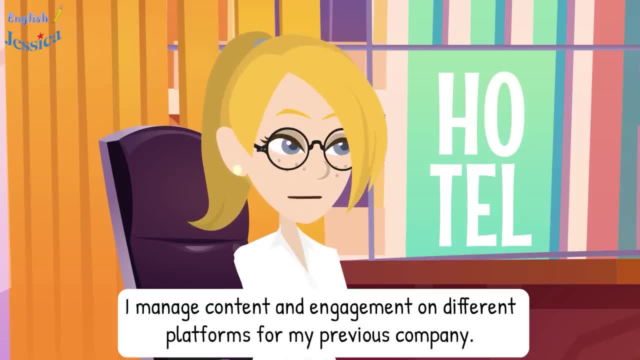 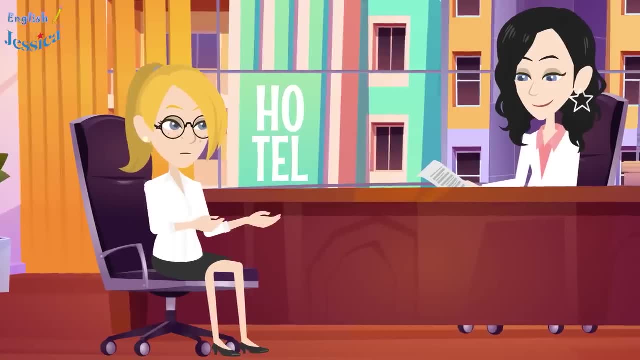 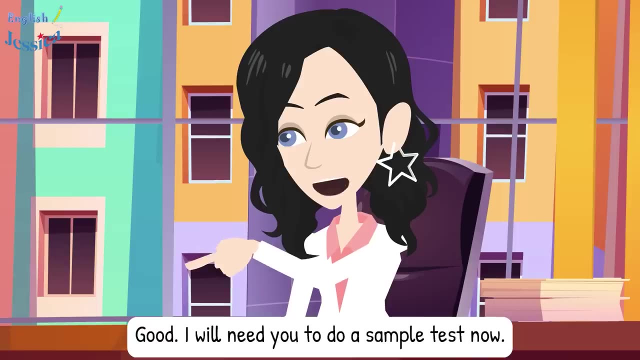 Yes, I do. I manage content and engagement on different platforms. for my previous company, Did you have to plan and create content or just manage? I mainly managed, but sometimes I had to do it also when the workload is huge. Good, I will need you to do a sample test now. Is it okay for you? 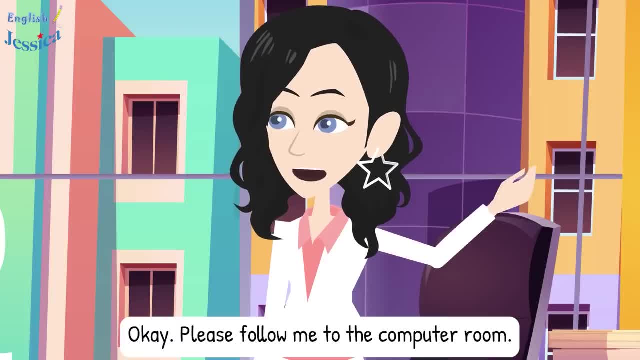 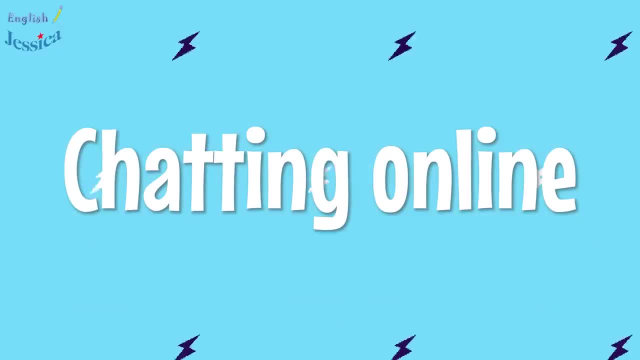 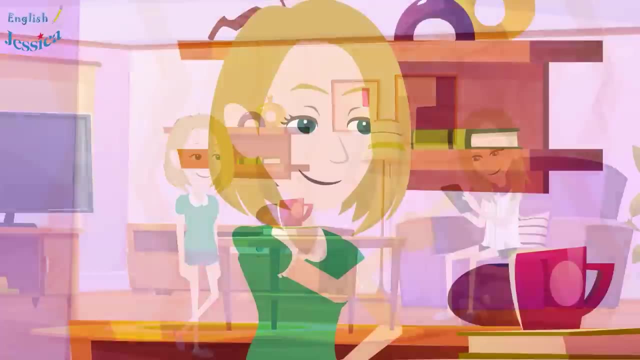 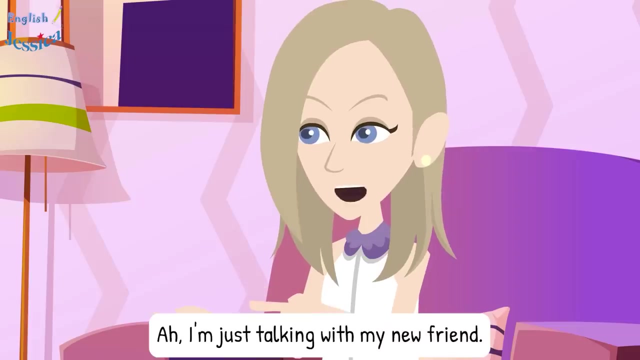 Sure, Okay, Please follow me to the computer room Chatting online. Who are you texting to Lily? Why are you keep smiling? Uh, I'm just. I'm just talking with my new friend. New friend, Very suspicious, Tell me. 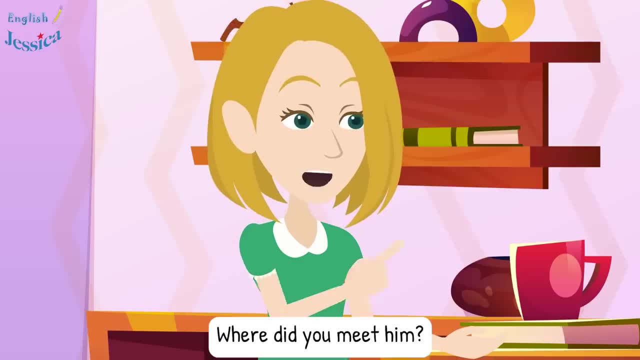 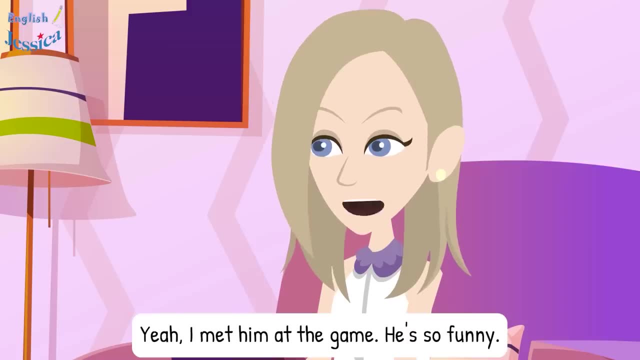 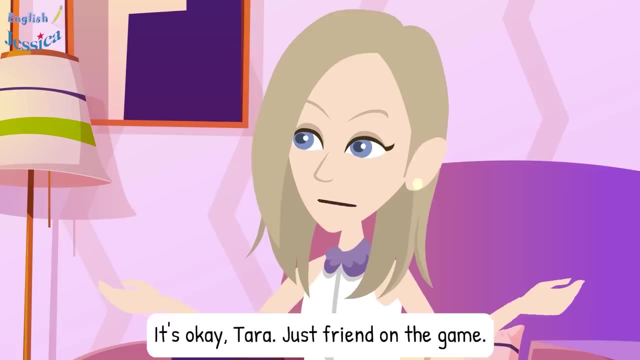 Tell you what? Where did you meet him? I haven't met him yet. What, Really? Yeah, I met him at the game. He's so funny. Have you seen his face? It's okay, Tara, Just friends on the game.